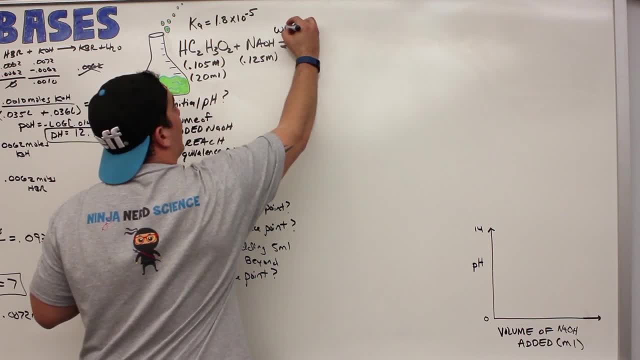 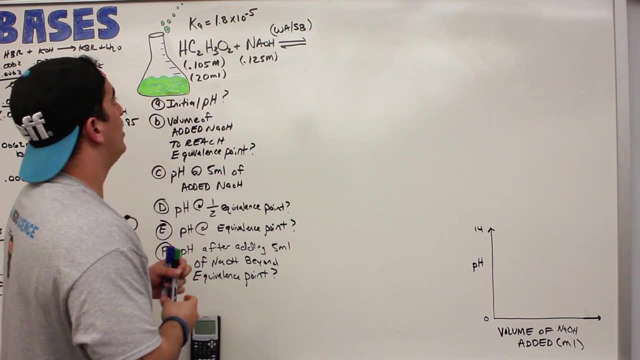 base. Now, in this one we're going to do, a acetic acid is a weak acid and then sodium hydroxide is a strong base. So that's, we're going to do a weak acid, strong base titration. So the first thing, 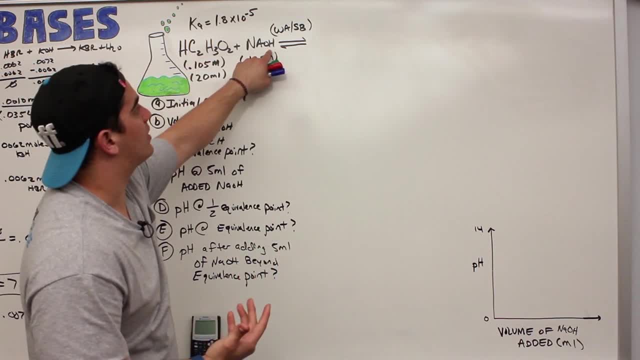 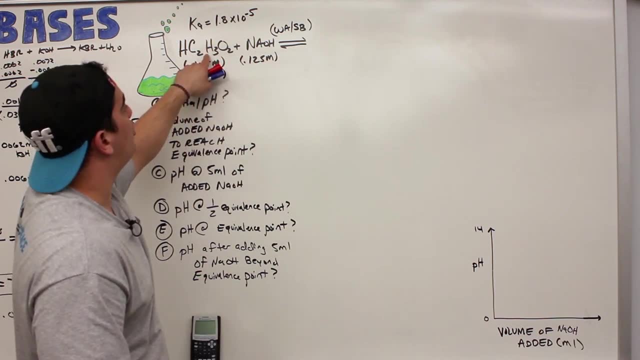 that happens is acids give up protons, So it's going to give up this H to that hydroxide. And what are you going to get out of that? You're going to get water. Sodium is going to be able to counter ion. this. what This C2H3O2, which is going to be the acetates? but he'll have a negative. 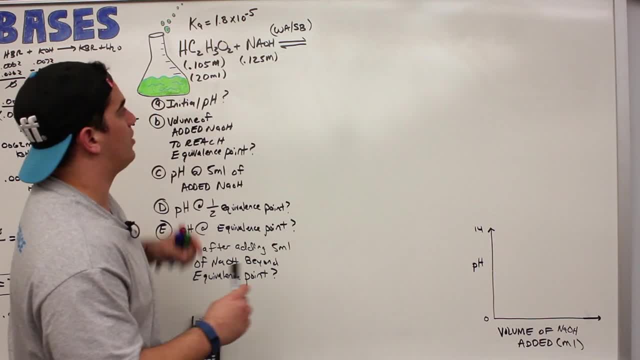 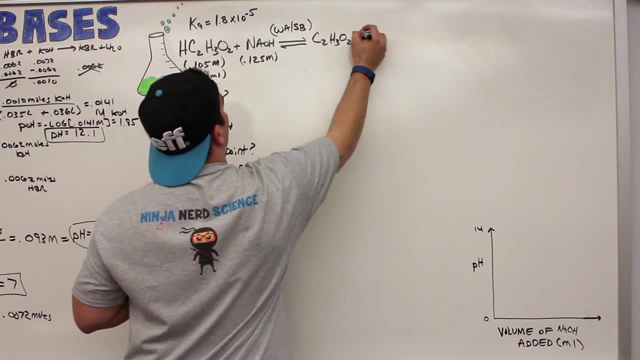 charge. But since sodium is a spectator ion, he dissolves in solution. So we're not even going to show sodium, We're just going to say we form acetate C2H3O2.. Negative. And then again the H combines with the hydroxide and gives you water, And then again. 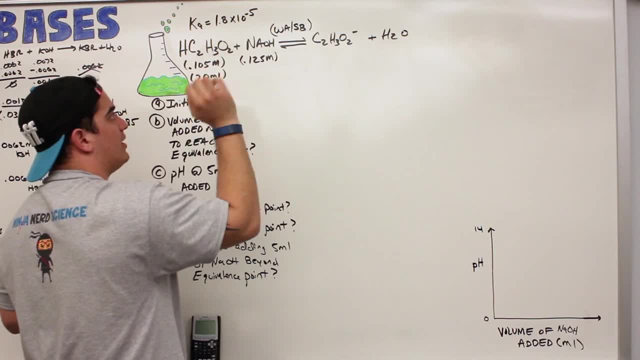 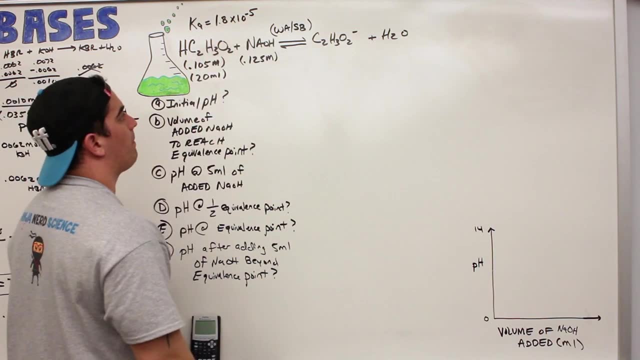 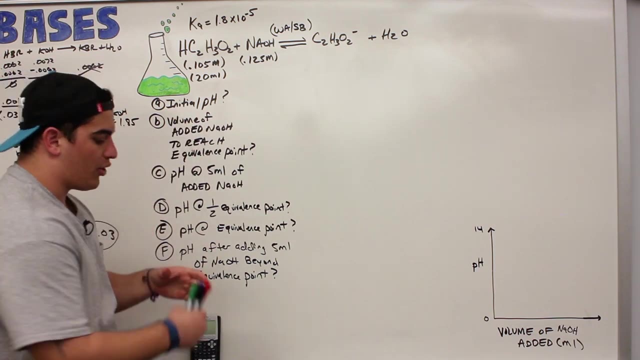 the Ka for this reaction, which means basically the acid ionization constant- how much protons are being given up over a certain period of time- is 1.8 times 10 to the negative five. All right, cool, So we're ready to start. The first question here says what is the initial pH. So I'm going to 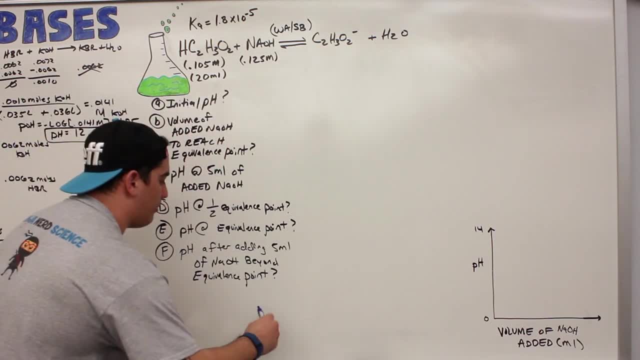 go back to that little beaker drawing I had. If you remember, I had a beaker sitting here and then in the beaker I had a beaker, And then in the beaker I had a beaker, And then in the beaker. 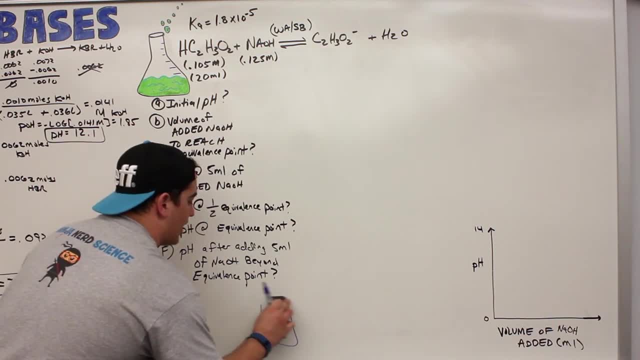 what did I have? I had the acetic acid. I have the acetic acid just kind of chilling in there just sitting there, All right. So what do I have in here? HC2H3O2.. He's just chilling in there, How. 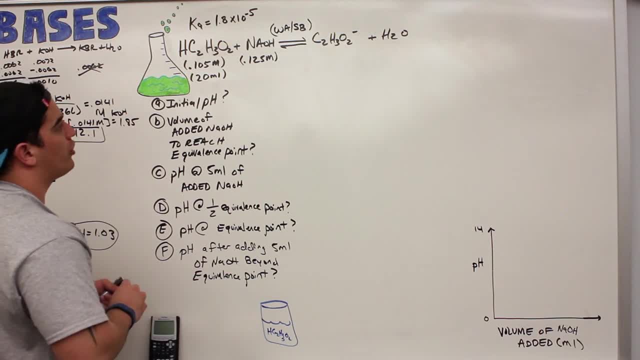 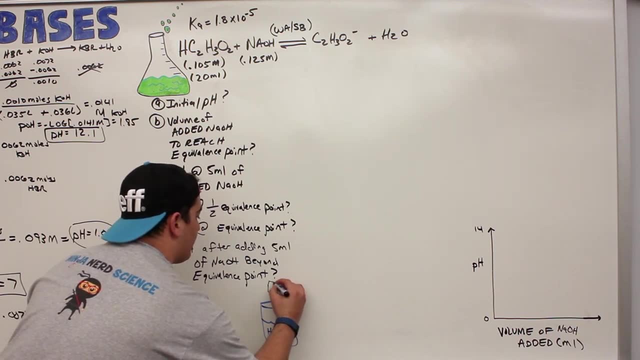 much of him. do I have in here? Well, I have a 0.105 molar, 20 mil sample here. And then what would I have here that I'm trying to drip in? I'm going to be dripping in what The sodium? 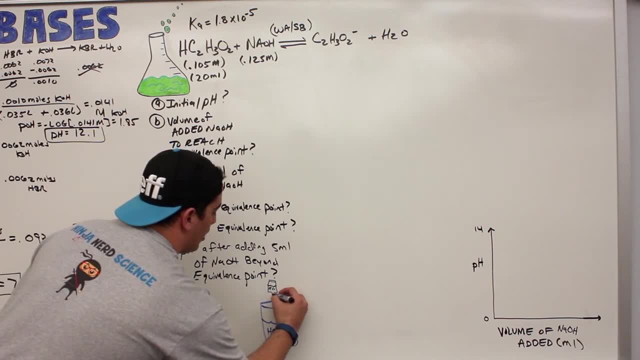 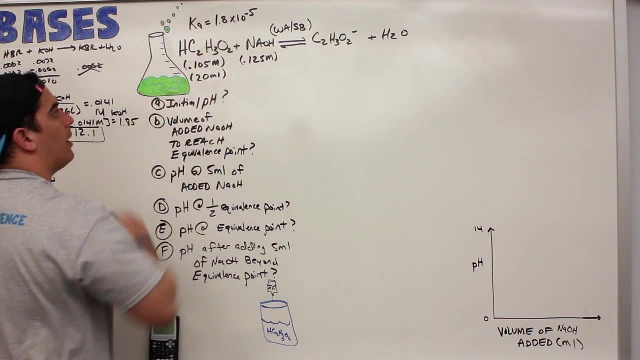 hydroxide. I'm going to be slowly dripping him in, All right, But they want to know. they want to know what's the pH of the solution before I add any sodium hydroxide in. So I'm only really looking at my weak acid. Remember the weak acid formula, guys? Let's write that sucker out. 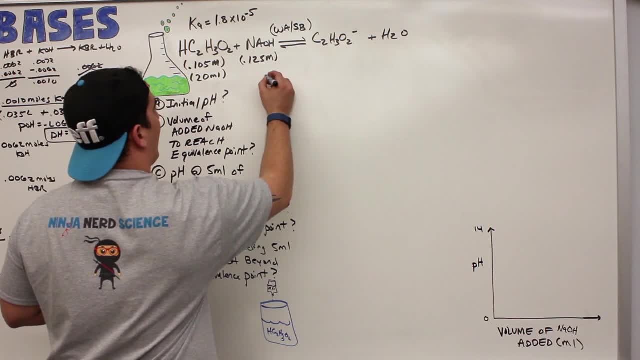 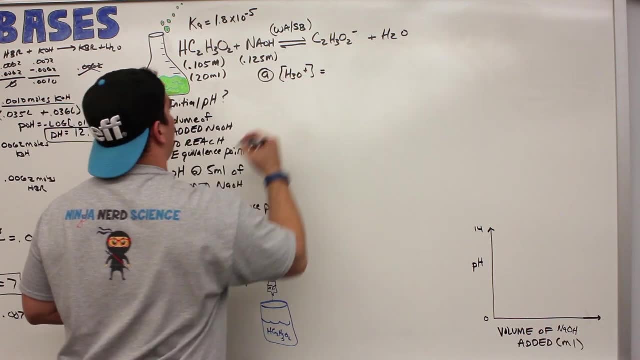 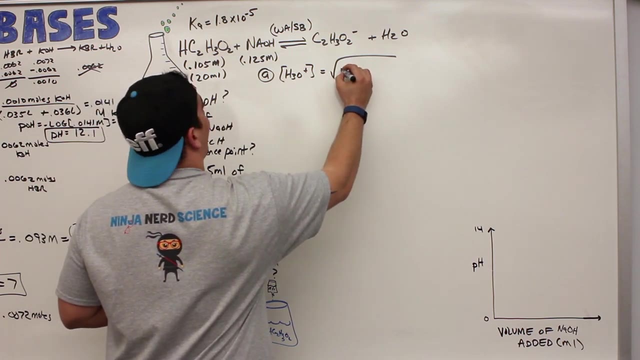 here. What is it So? start here with A right. here We say: H3O plus concentration is equal to the square root, And the only reason we use this one is because this is our weak acid formula is equal to the Ka. What's our Ka? 1.8.. 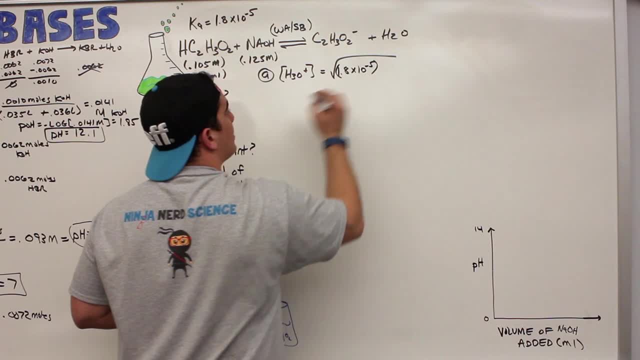 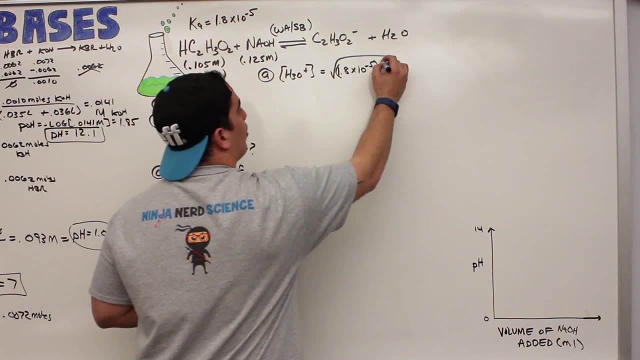 Times 10 to the negative 5, right Times, the concentration of our weak acid, which is HC2H3O2, which is a 0.105 molar solution. And again, we assume that that X because we would subtract X. 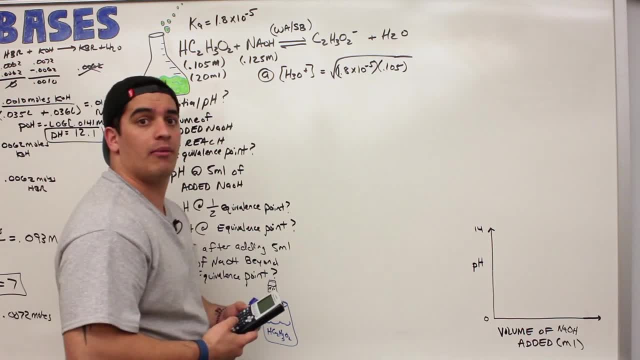 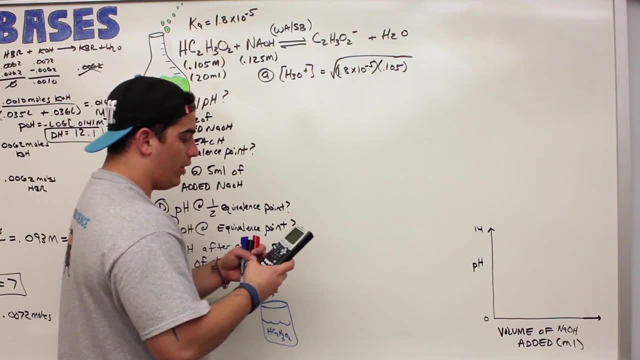 right, We're going to assume that that is zero, but we'll check it by using the 5% rule, right? So what do we do? 0.105 times 1.8? second E to the negative 5.. And then I'm going to. 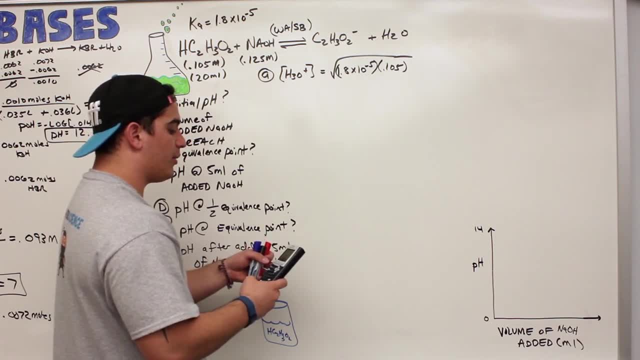 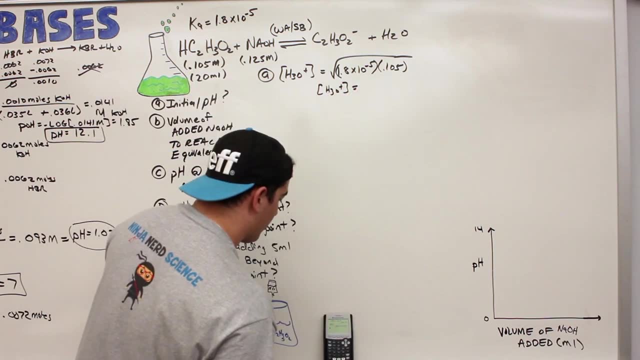 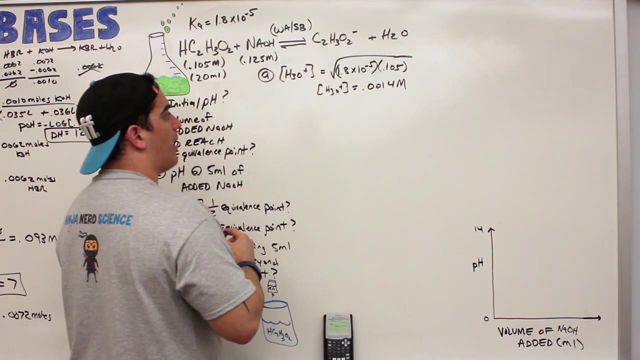 square root, this MOFO, and I get 0.0014.. Let's write that puppy down. So out of this H3O plus concentration, I get 0.0014 molarity. Well, what do I do now I do? pH equals the negative log of. 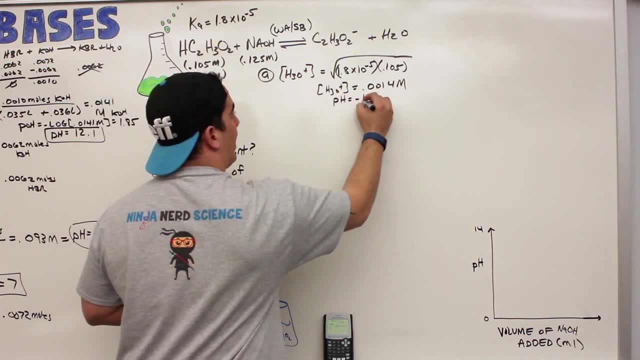 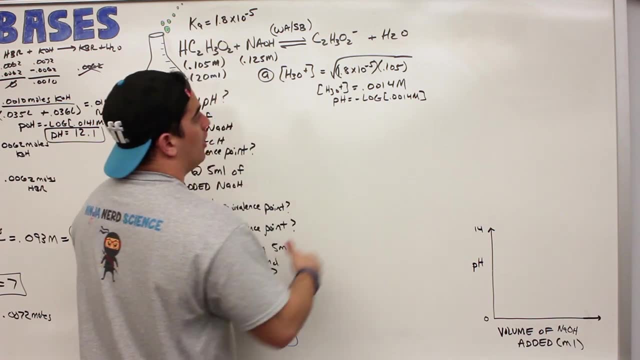 that, because that's our formula, pH is equal to negative log of 0.0014 molarity. What's that going to give me? Okay, so 1,, 2, 3.. So it's probably going to give me 0.0014 molarity. 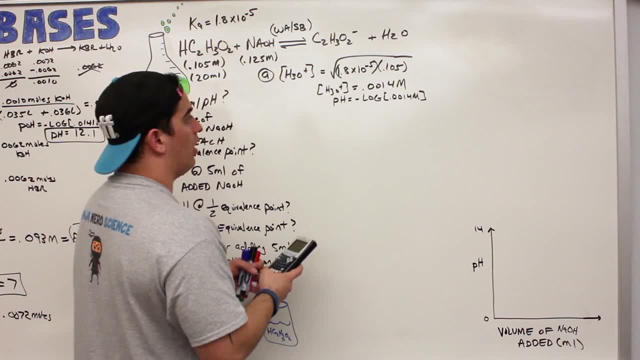 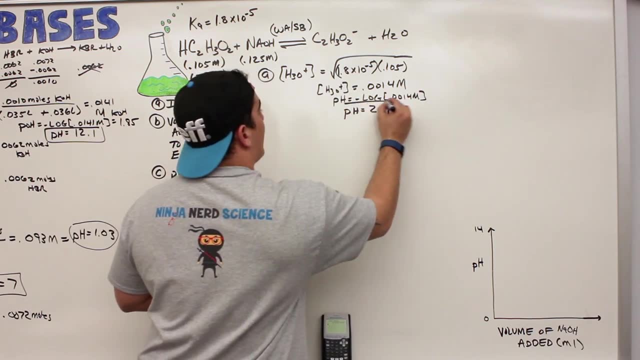 It's probably going to give me somewhere in between, like 2 point something, right? So negative log of 0.0014 pH is equal to 2.9.. Okay, so that is the answer for the first one for part A. 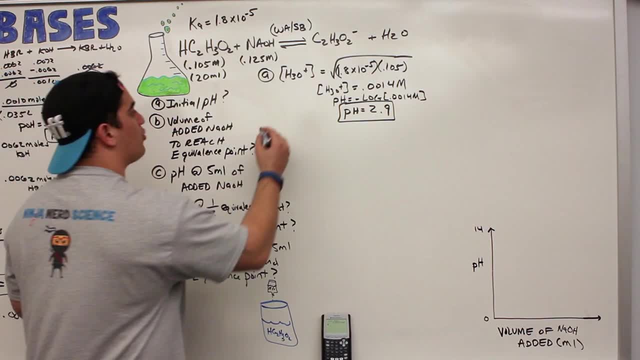 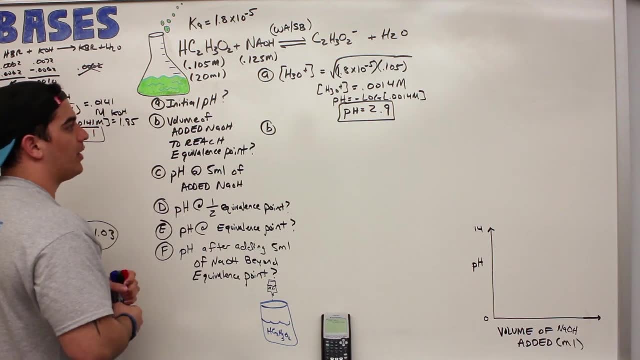 Second part, part B, it is how much volume of sodium hydroxide needs to be added in order for this to be able to reach the equivalence point. What was that formula for the equivalence point That the moles of the acid acetic acid? 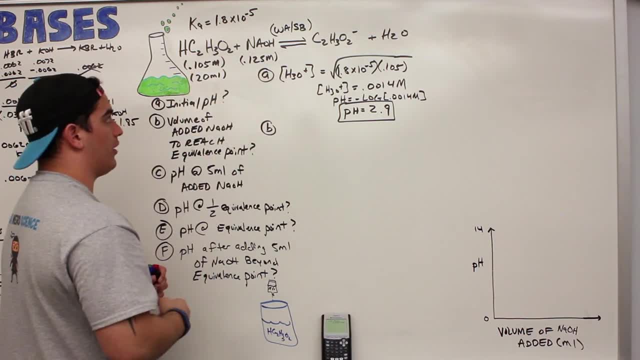 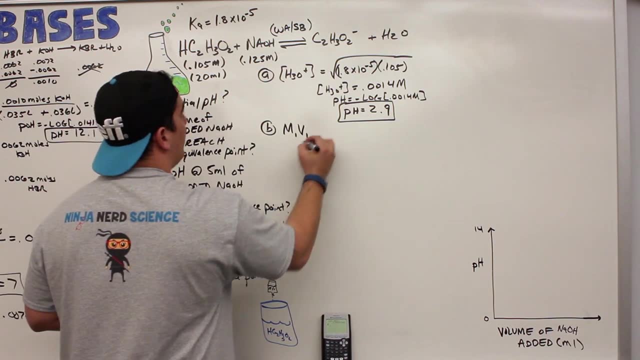 and the moles of the base sodium hydroxide have to equal each other. What did we use for that formula? if you remember, We took M1,, which is going to be the acetic acid times, V1,, which would 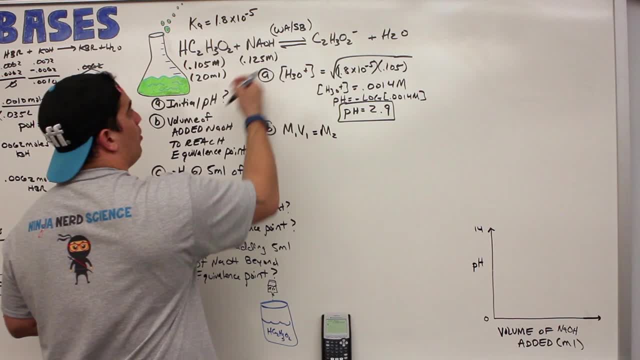 be, the volume of the acetic acid equals M2, which is the molarity of our sodium hydroxide times V2, which we don't know. so we're trying to figure out and we're going to go ahead and rearrange. 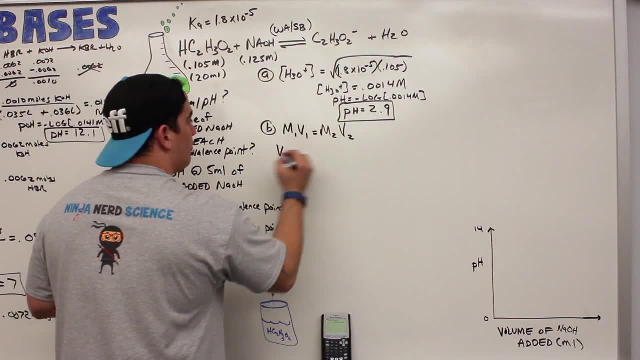 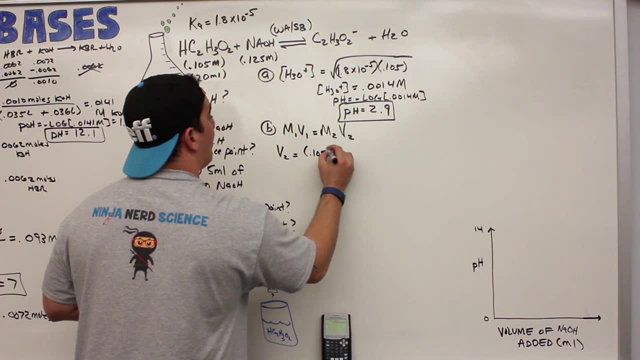 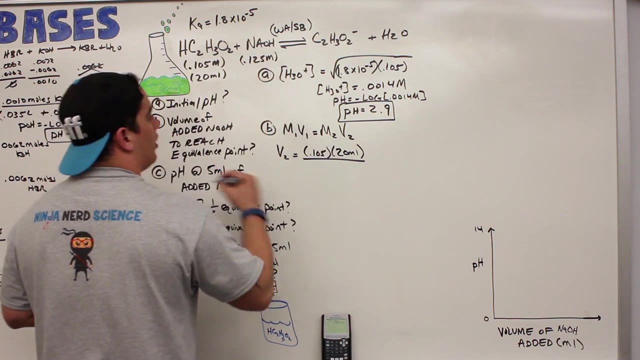 to solve for V2.. So V2 is equal to the molarity of HC2H3O2, which is going to be 0.105 times its volume, which is 20 milliliters all divided by the molarity of our sodium. 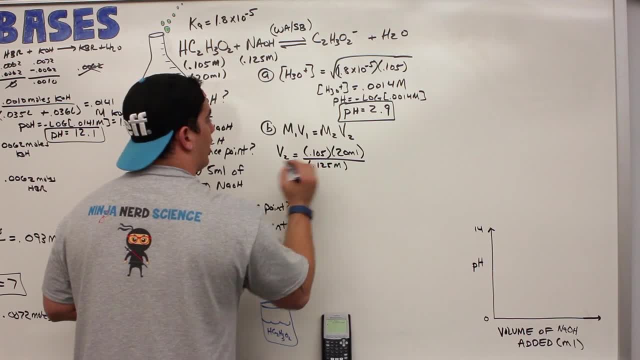 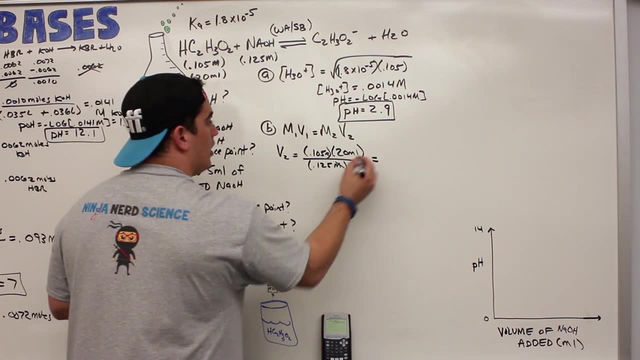 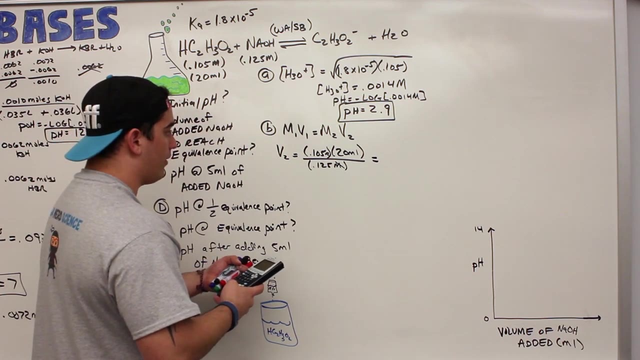 hydroxide, which is 0.125 molarity. right, And this will be molarity also. Keep my units together and then the molarity will cancel out and I'm going to get a volume out of this. What's that volume? Let's see 20 times 0.105 divided by 0.125, and I get. 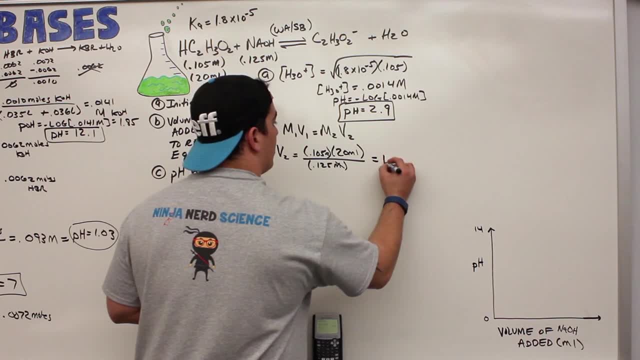 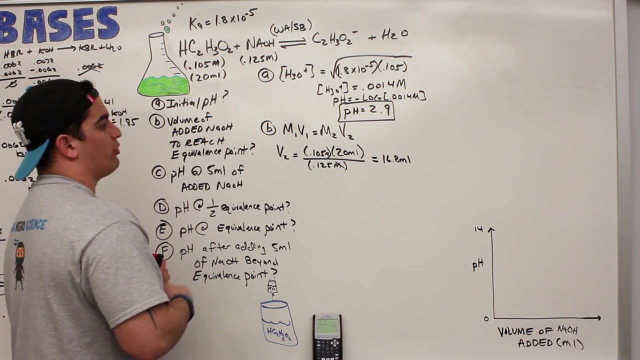 16.8 milliliters. So 16.8 milliliters of sodium hydroxide is needed in order to be able to get us to the equivalence point, and that should actually make sense. Why? Because this is a weak acid. 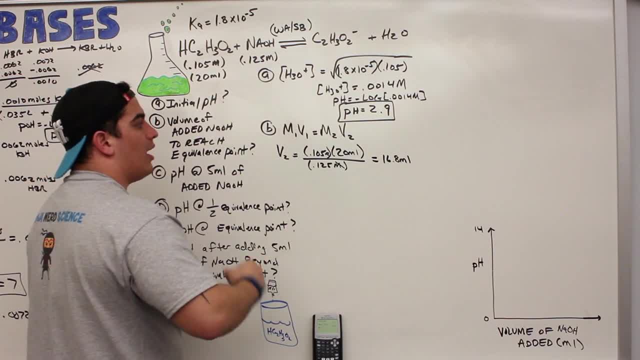 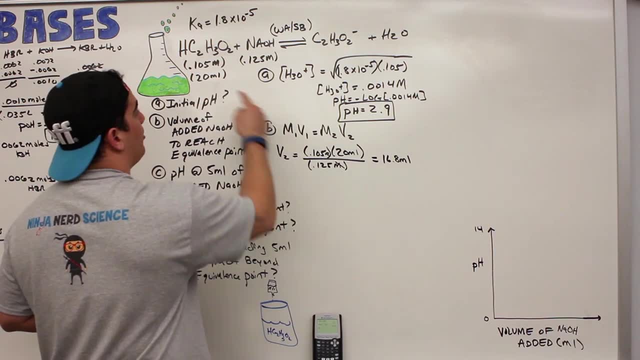 That's a strong base. I shouldn't need more sodium hydroxide to be able to get me to the equivalence point. I should need less volume, because he's so strong it wouldn't take much volume of him to be able to bring him to the equivalence point. That should make sense. Okay, so he is the. 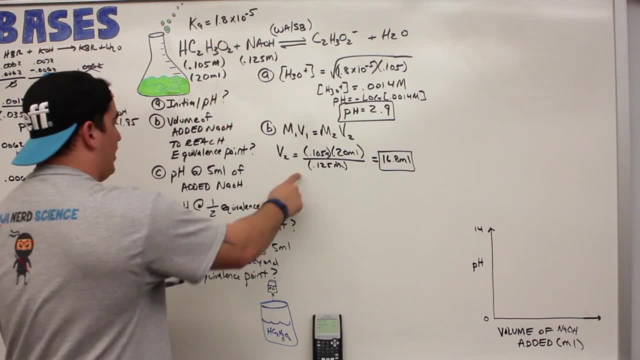 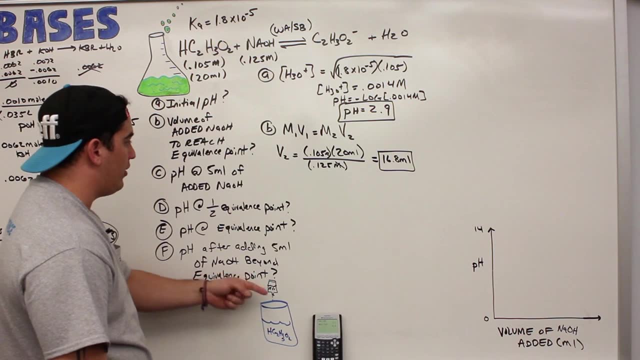 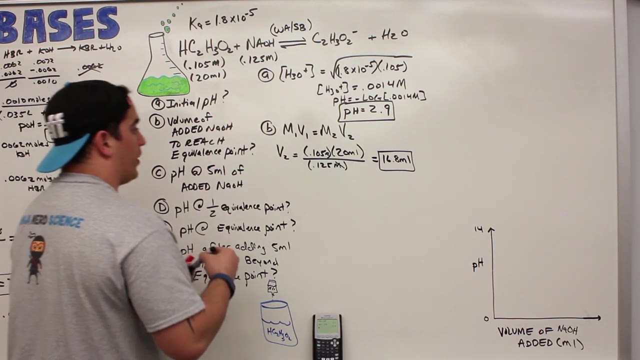 volume that's needed to be able to get us to the equivalence point. We're going to need that soon. Let's do part C. Part C says what's the pH after you drip in. you start titrating and adding in 5 milliliters of sodium hydroxide. Let's write out this equation here, because we're going to need it. 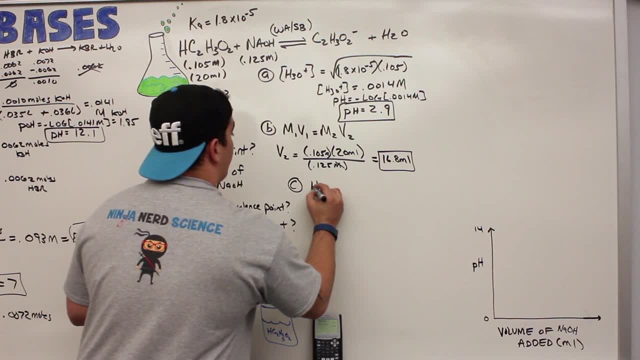 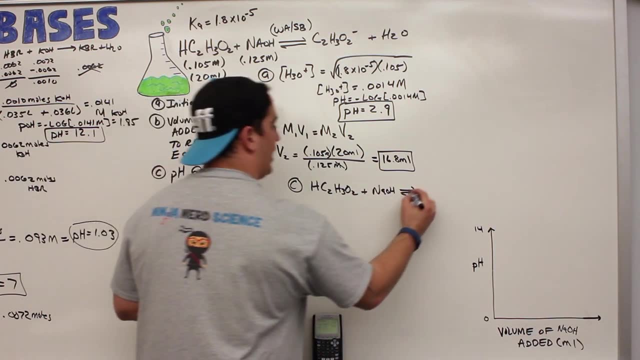 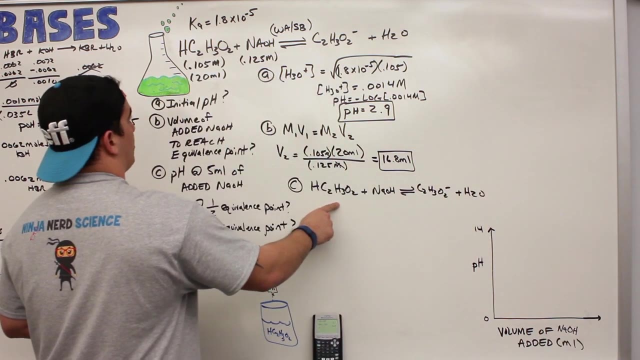 for part C. So what is it? We have HC2H3O2 plus sodium hydroxide and again equilibrium reaction, H3O2 negative and water. What was the starting? moles. Well, how do we get moles? I take the volume. 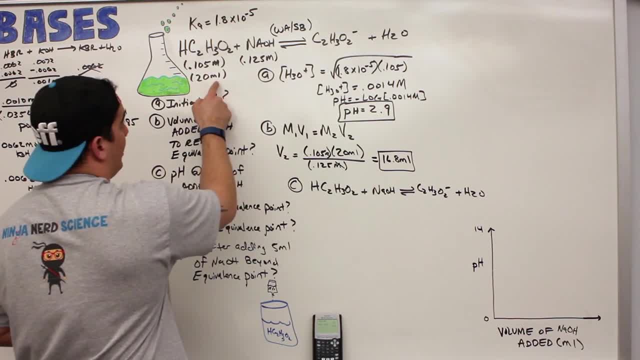 of this acetic acid, and I'm going to get it into liters and then multiply it by the molarity. What do I do then? Let's actually do that. Let's write that out quick. So 20 milliliters, which we 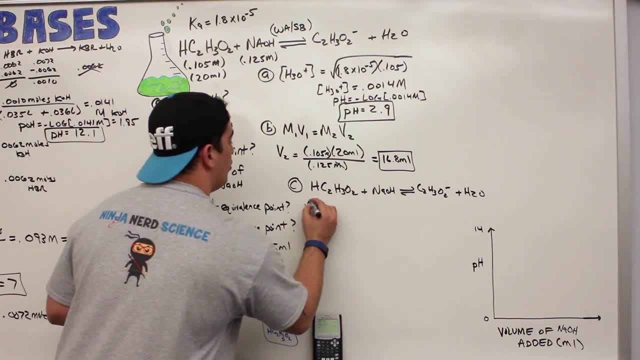 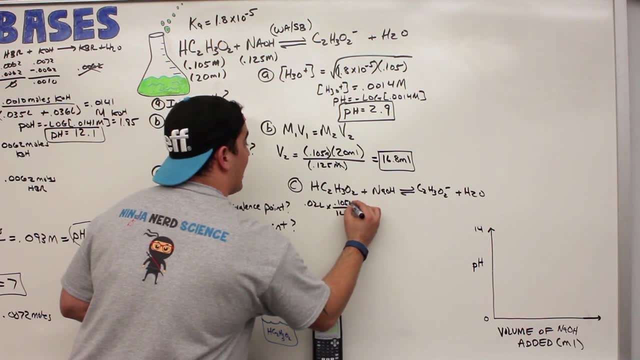 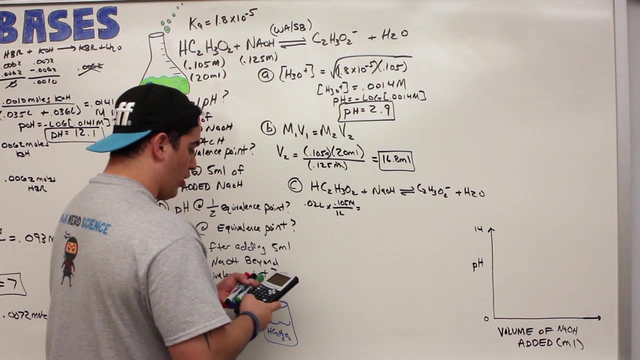 can just get that into liters. You divide it by 1,000, so that's 0.02 liters times that by 0.105.. And what would I get out of that? I would get my moles of acetic acid. What's that? Let's see, We have 0.105 times 0.02, and that is. 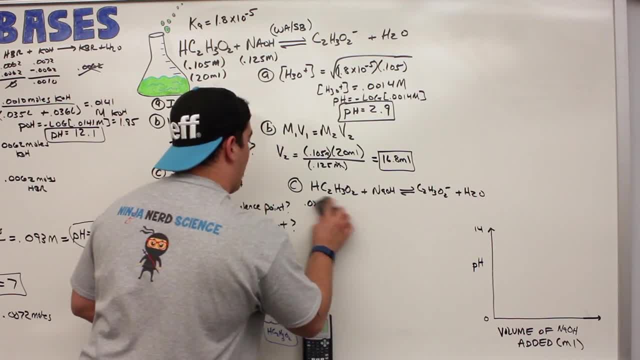 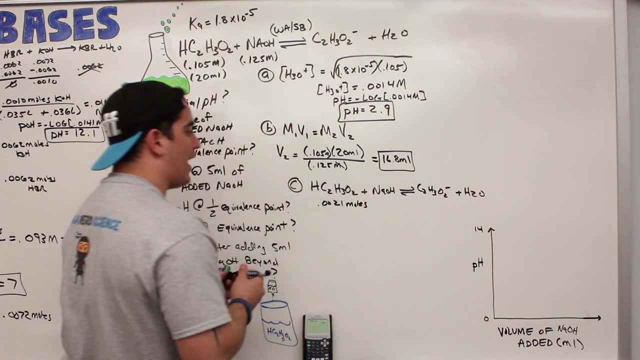 0.0021 moles. I'm going to write that down now. So I have 0.0021 moles, So 0.0021 moles of acetic acid sitting there. Then I'm going to take and add 5 milliliters of sodium hydroxide. So I'm going to 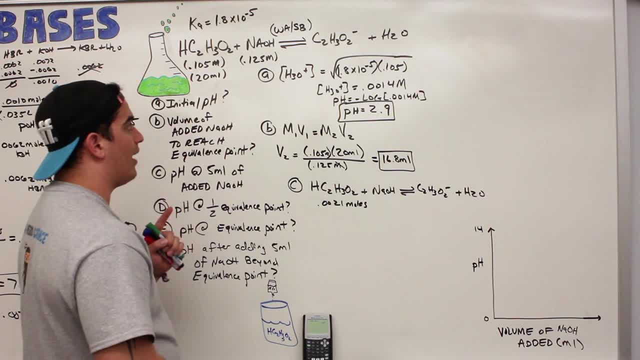 do the same thing. I'm going to get this into liters, which is 0.005 times 0.125.. What's that give me? So, again, I'm going to get my moles of acetic acid and I'm going to write that down. now. 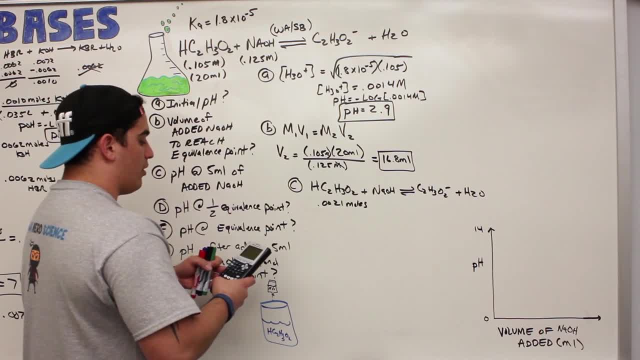 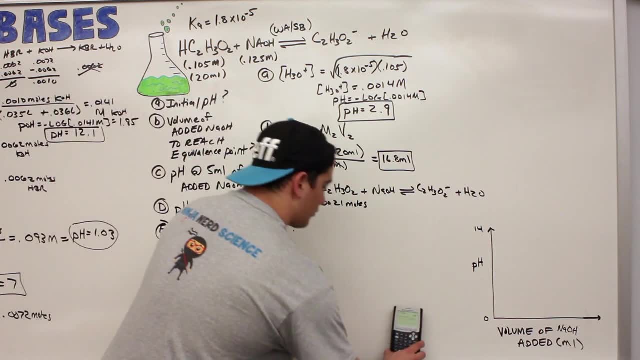 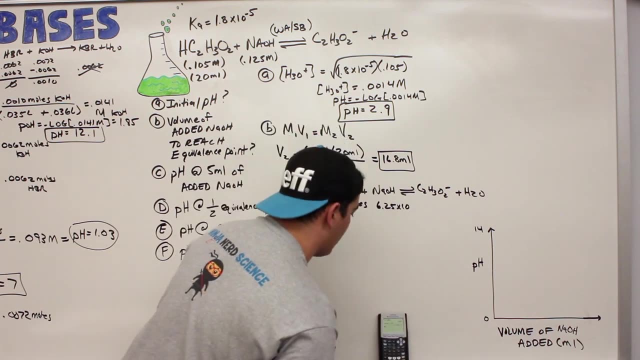 Take your 5 mils, divide it by 1,000, and that'll give you 0.005, and then multiply that by the molarity, which is 0.125. And you get 6.25 times 10 to the minus 4 moles. Beautiful, Now what? 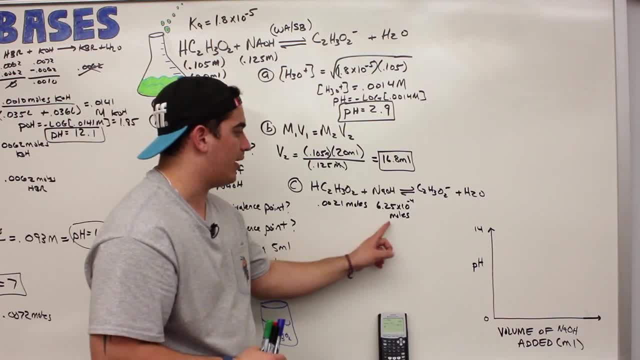 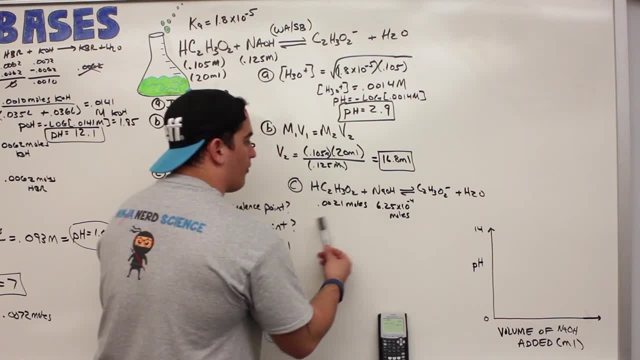 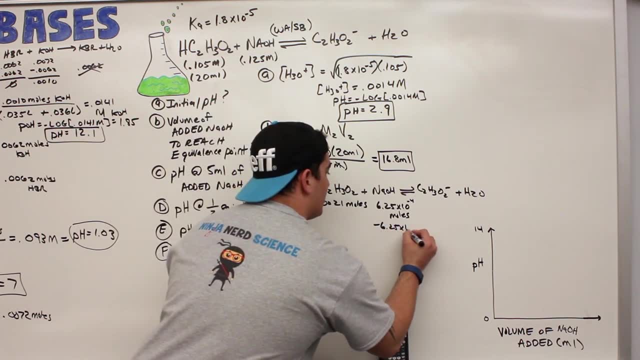 So what do I do here? I subtract this one from this one because I'm going to use up all of him and react it with this guy. So I subtract 6.25 times 10 to the negative 4 moles of the sodium. 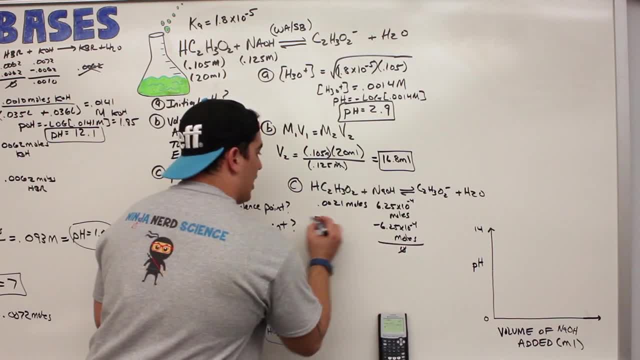 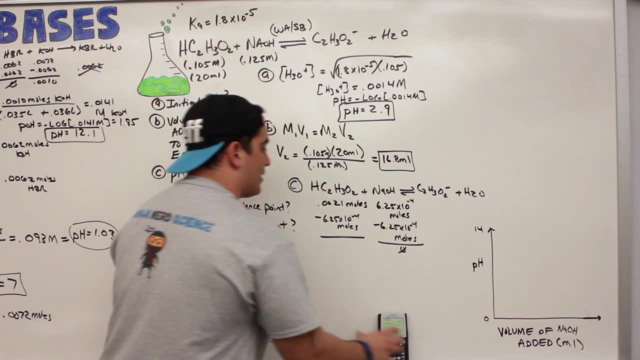 hydroxide and if I react all of him, it'll be 0. And I'm going to subtract from him 6.25 times 10 to the minus 4 moles. but I'm not going to use up all my acetic acid. I'm going to have some acetic. 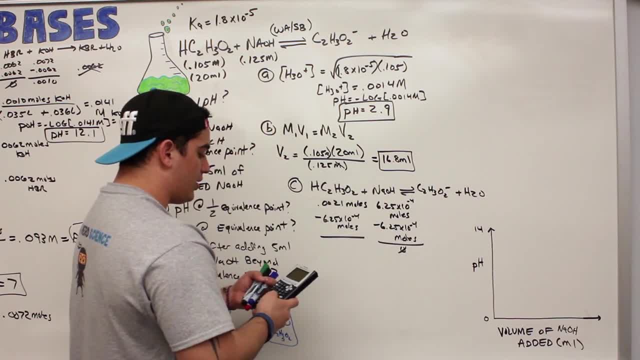 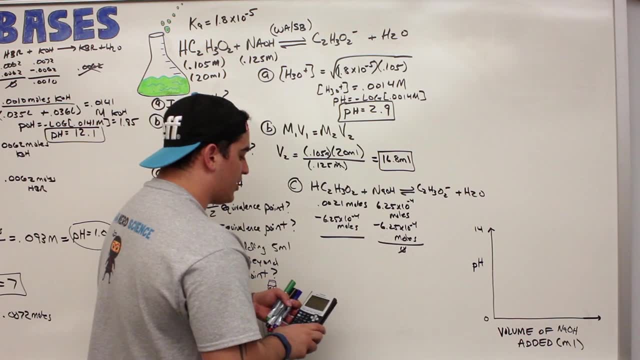 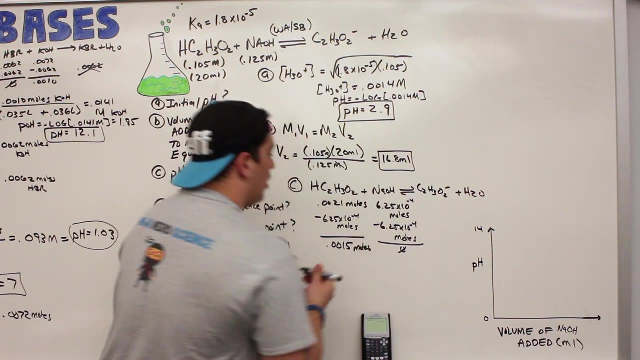 acid left over, hopefully right. So I do 0.0021, subtracting it from 6.25 times 10 to the minus 4 and I get 0.0015.. So let's write that down: 0.0015 moles, But 6.25 times 10 to the negative 4 moles. 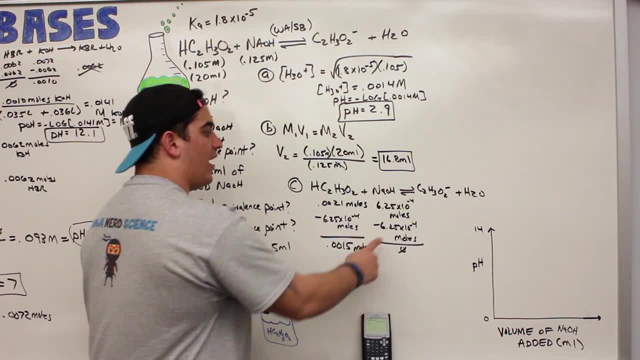 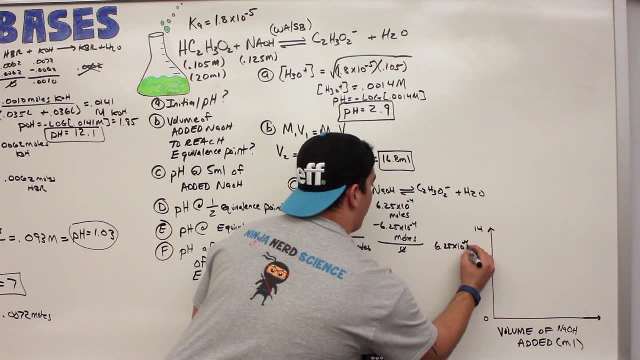 of him, reacted with 6.25 times 10 to the negative 4 moles of him and produced 6.25 times 10 to the negative 4 moles of this guy, which is what I get. So I get 0.0015.. So I subtract 6.25 times 10 to the. 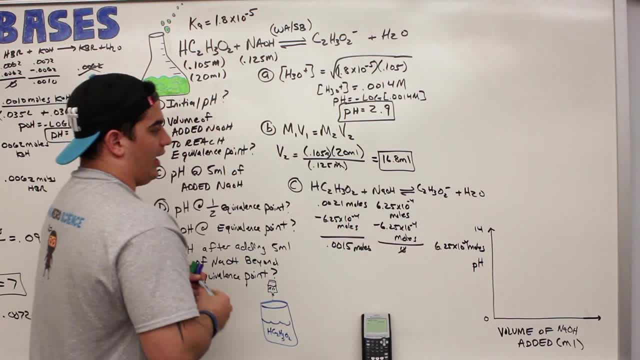 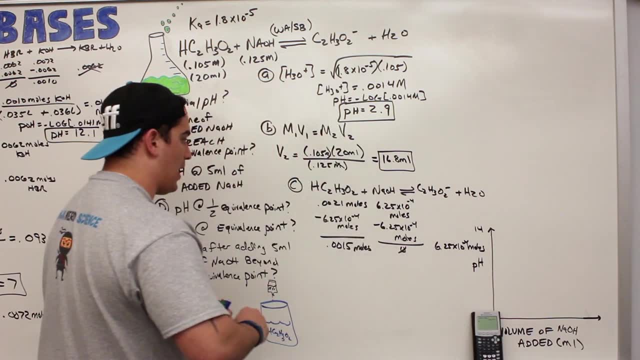 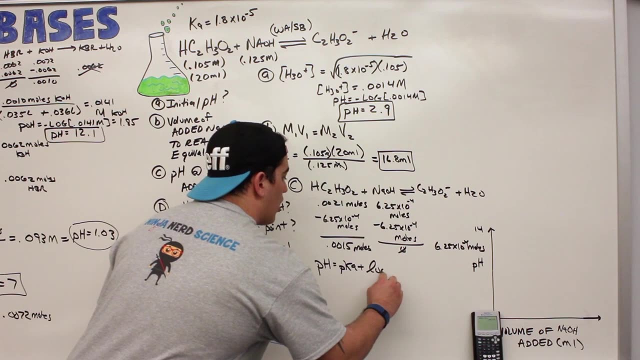 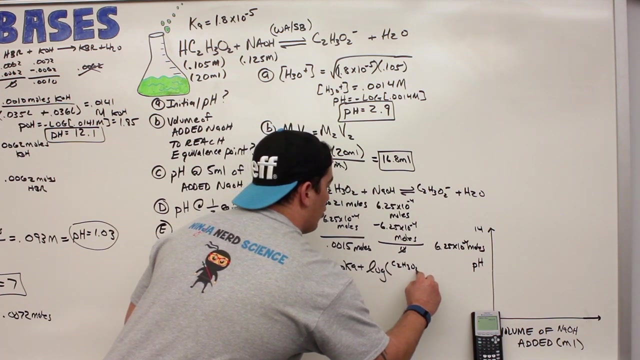 negative 4 moles of him and produced 6.25 times 10 to the negative 4 moles of him. Now I get the Schülerünungluke, the club of the answer project here. What we go to packaging 0.0025. 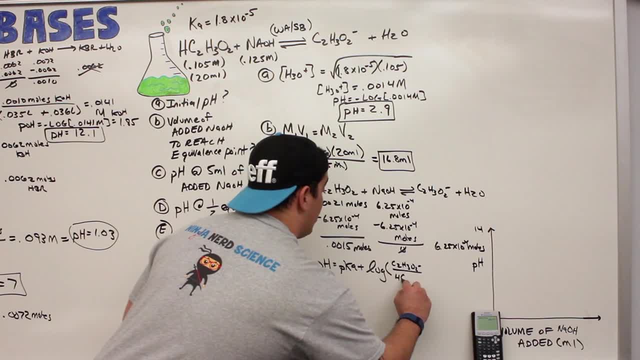 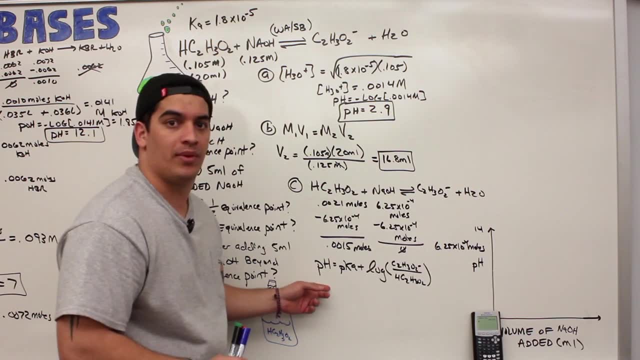 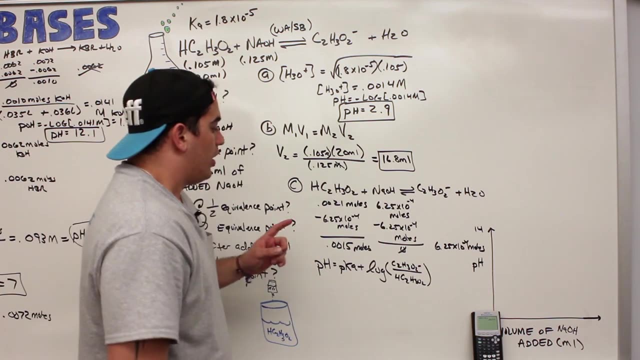 is weak acid, in this case, which is hC2H3O2, and what do I get there? Boom, I have my Henderson-Hasselbalch equation. This is beautiful when you're doing this with certain types of buffer equations. This is our nice little buffer equation, So. 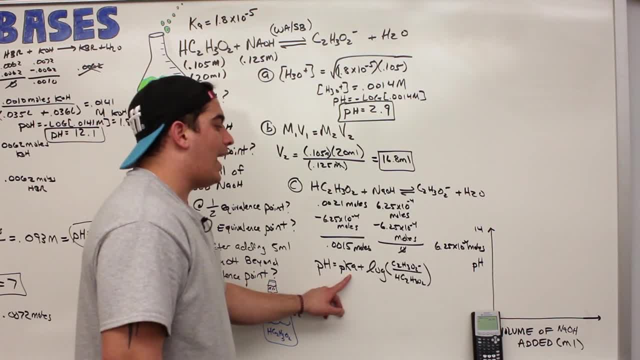 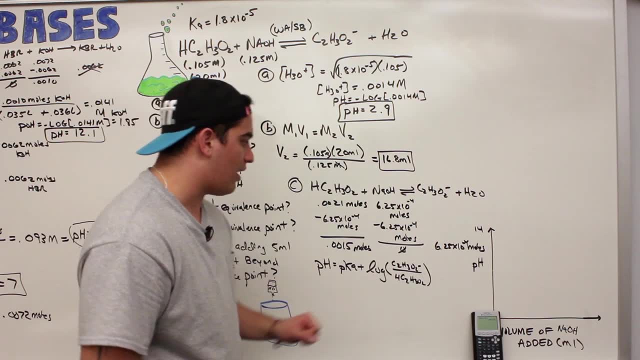 now, if you remember from the intro video, we talked about the term pKa, and pKa was what It was: the negative log of the Ka. So in order for me to start filling all of this stuff in, alright, here's one more thing, Because I'm going to take. 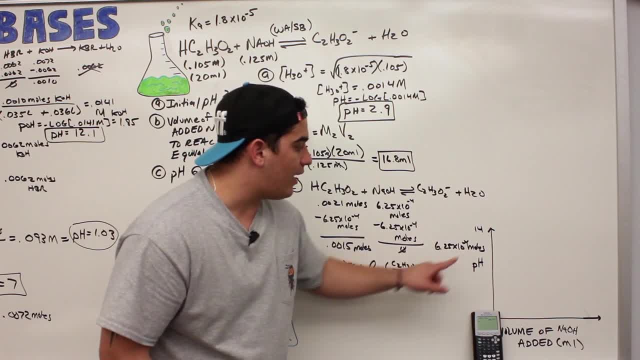 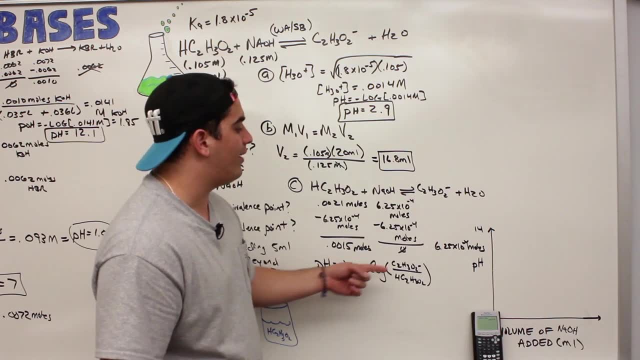 0.0015 moles. I'm going to plug it in there. 6.25 times 10 to the negative 4 moles: I'm going to plug it in here. What did I just say before? I needed a concentration. right, I need a molarity. I could go ahead and divide this by the. 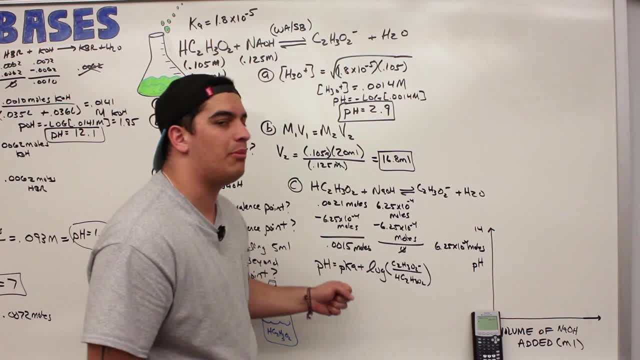 total volume at that point right there, each one of them, but it's going to be the same number ratio, So I don't need to do that. So I'm just going to keep them in moles so that I don't have to waste time here. So what am I going to do then? 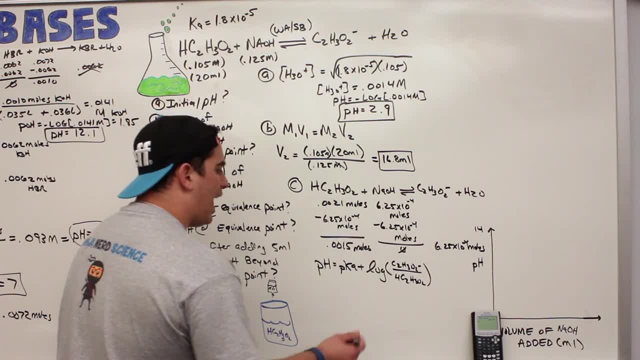 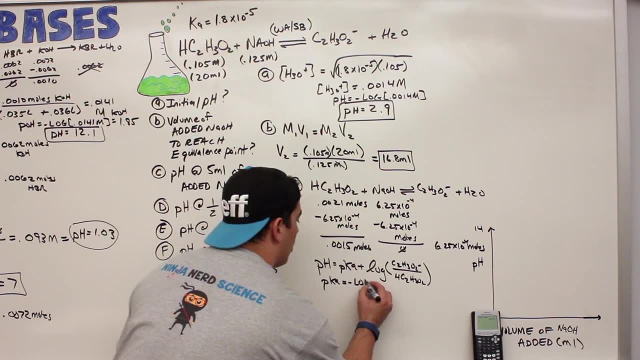 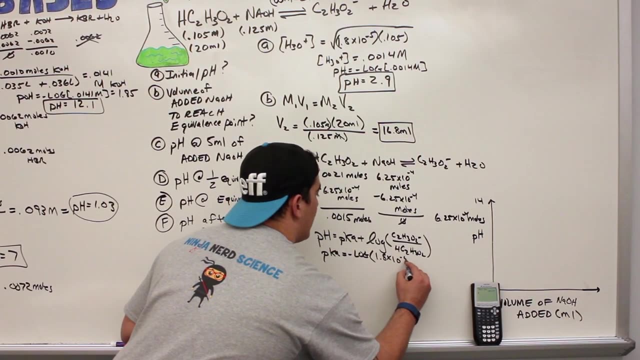 Let's go ahead and plug some of the stuff in and I'm going to show you how we get pKa Actually. now I'm going to show you pKa first. So pKa, as we said, is equal to the negative log of the Ka. What was our Ka? Our Ka was 1.8 times 10 to the negative. 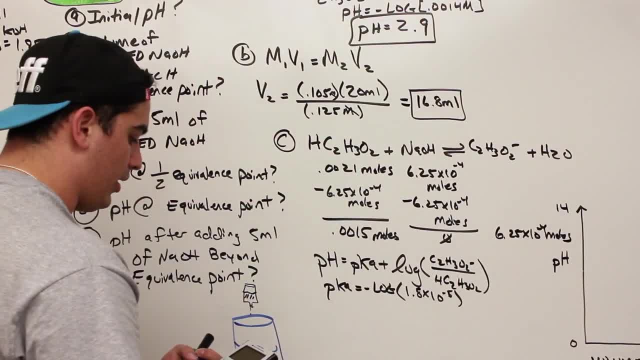 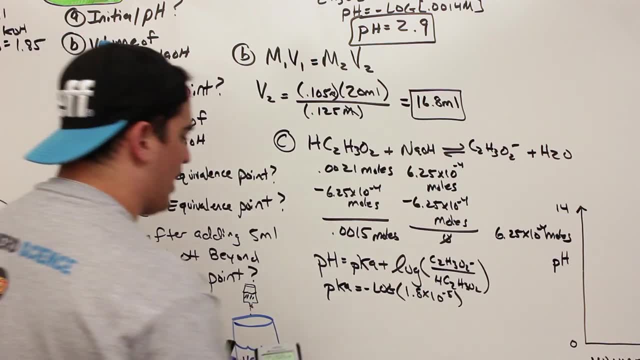 5.. Let's plug that in. It's going to be like 4 point, something, right? So take the negative log of 1.8, second e to the negative 5 guys and we get 4.74.. So what do we get? 4.74.. 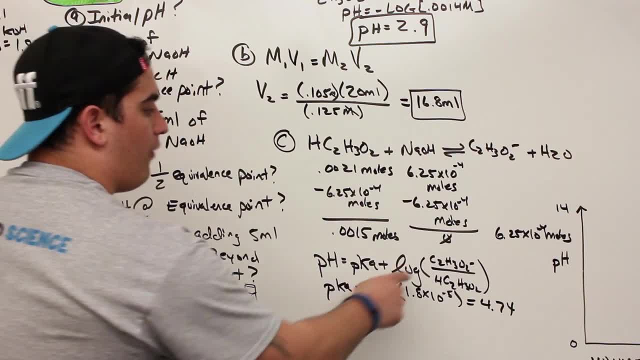 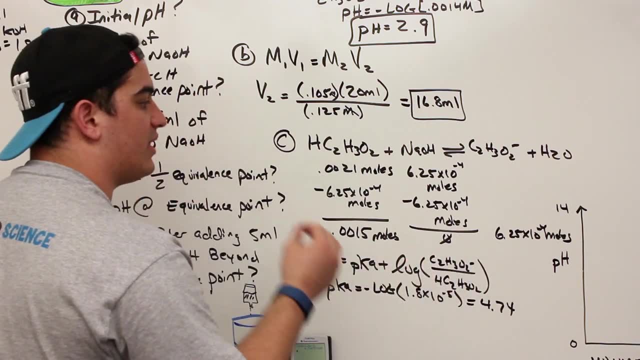 So now we have our pKa, We have our acetate molar amount right there and we have our acetic acid molar amount, And we can keep them in moles because it's going to be the same ratio if I divide both of these by the same volume. Don't need to do that, Let's plug. 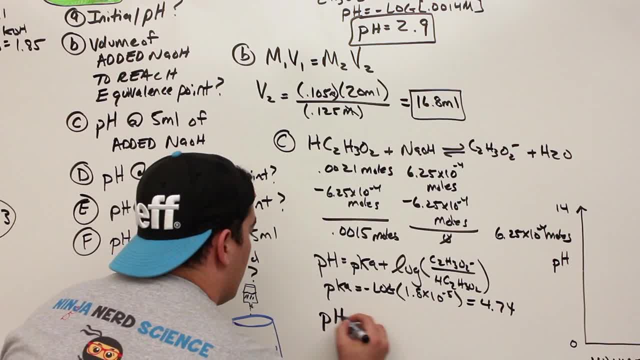 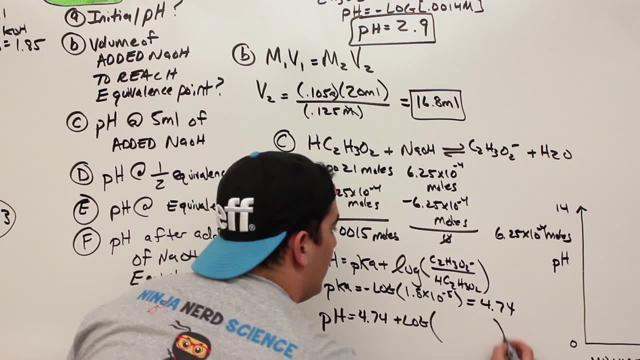 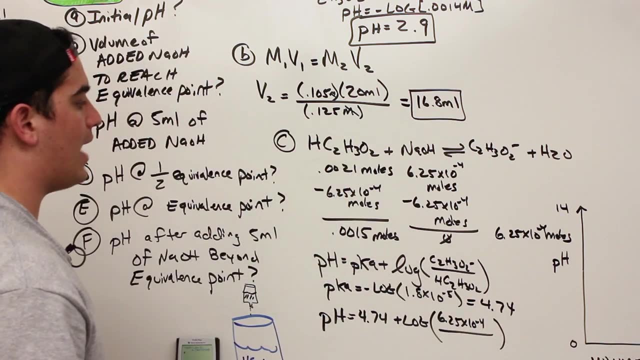 it all in. So pH is equal to pKa, which is 4.74, plus the log of the moles of my base, which is 6.25 times 10, to the minus 4.. So pH equals 4.74 over the moles of my acid, which is .0015 moles. Let's plug this puppy. 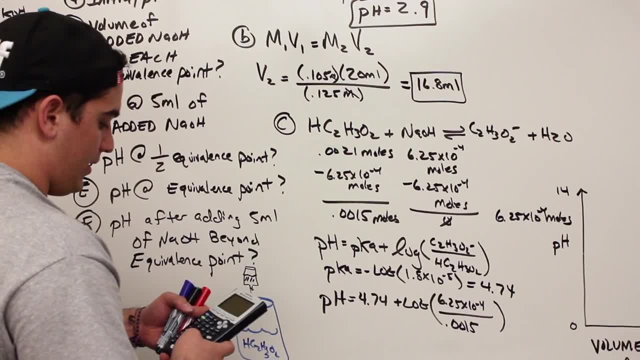 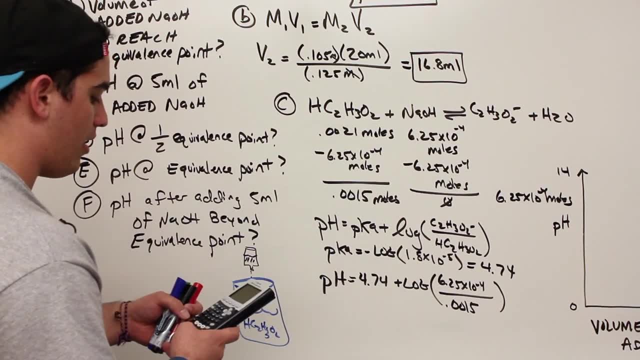 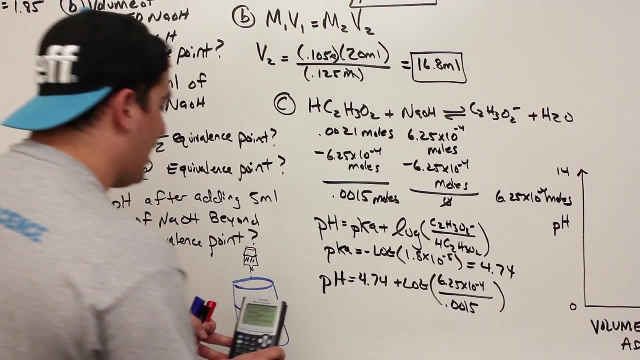 in and see what we get. So we take 6.25, second e to the negative, 4, divided by .0015, and then we're going to take the log of that number, guys, and then we're going to add that to 4.74 and I get a pH of 4.36.. 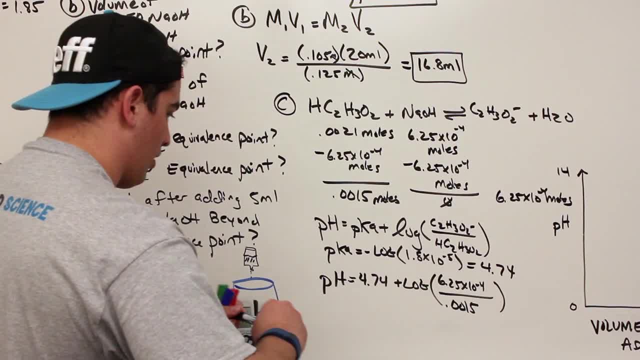 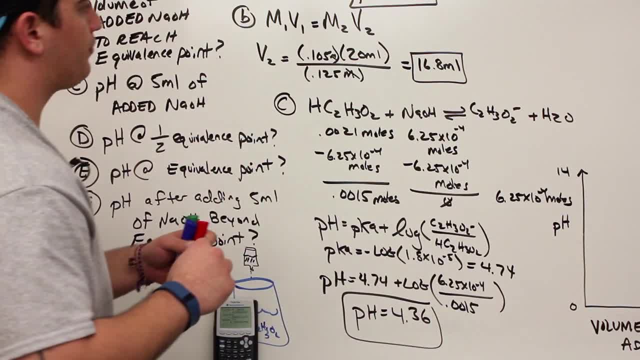 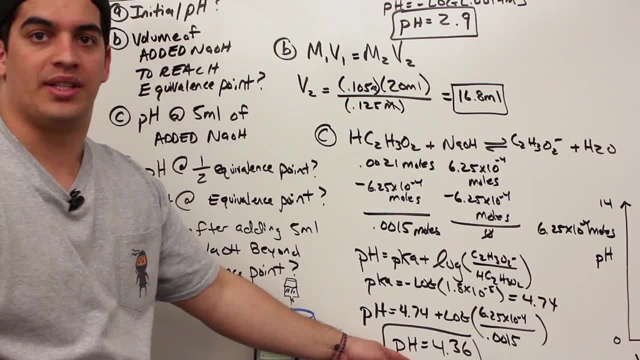 We added in 5 mls of sodium hydroxide and our pH went up to 4.36.. That should make sense, because we added base. All right, cool, That one was a little bit tough one, right? Let's move on to the next one. 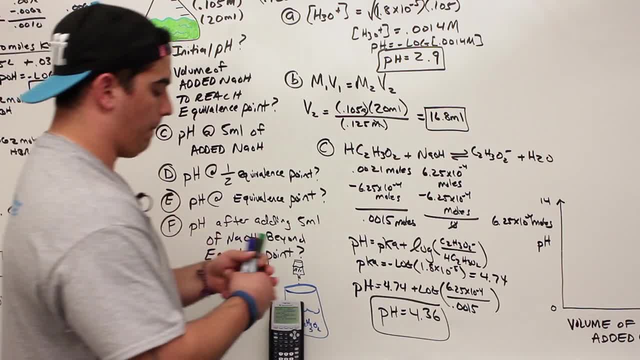 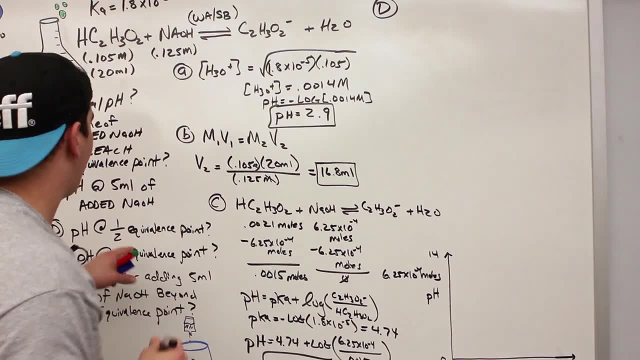 Oh, we get a little break here. Ah, we get a little break here, because this one's really easy. d Okay, so D says: what is the pH at half the equivalence point? Well, at half the equivalence point, what does that mean? 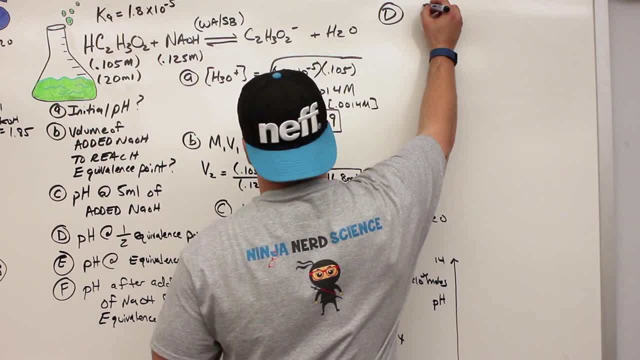 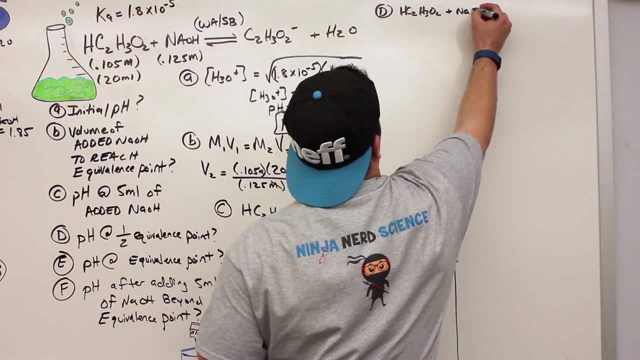 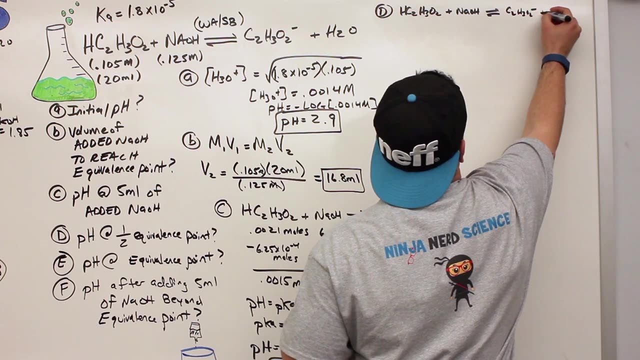 Okay, let's come over here. Let's say I wrote out over here C2H3O2 plus sodium hydroxide. What does that give us? That gives us again C2H3O2 negative and water right. 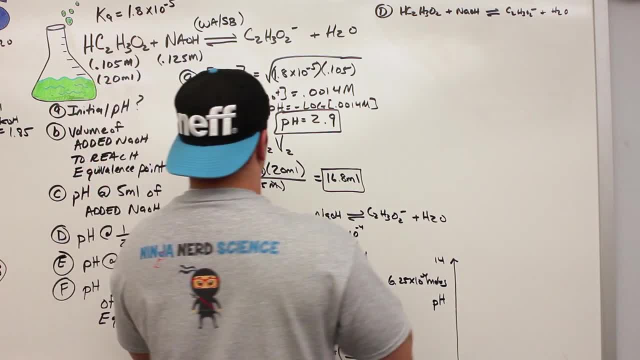 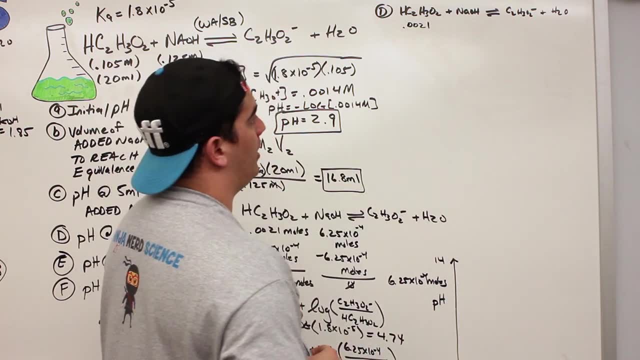 Now, what was the moles that we had for this C2H3O2? We had .0021.. Now, at half, the equivalence point means that there's a certain volume that we need to be able to get us to this point. 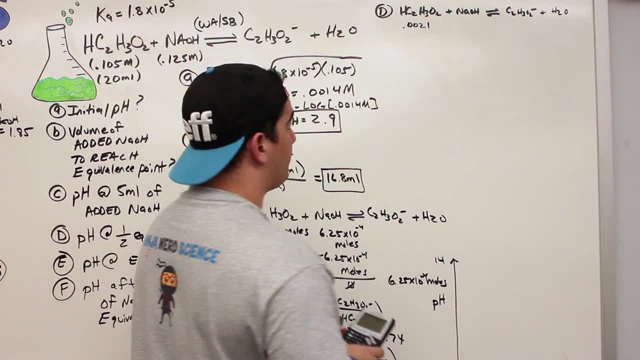 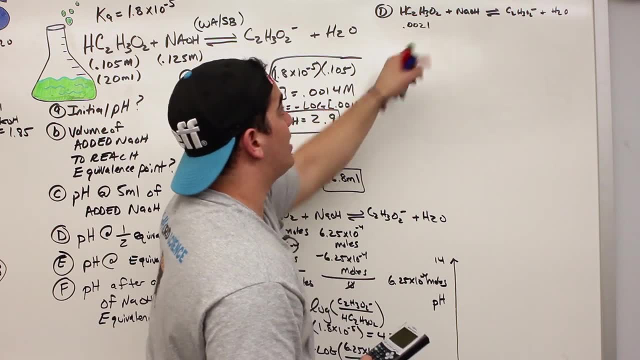 But basically this is what it means. If I take .0021, I'm going to figure out what half of this moles is, Because I'm going to get half the equivalence point. So what does that mean? then? Let's say I take .0021 and I divide that by 2.. 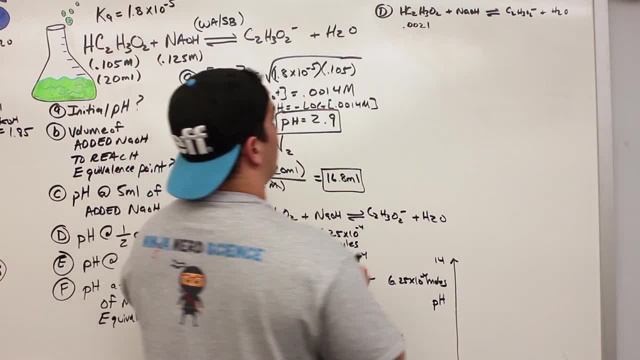 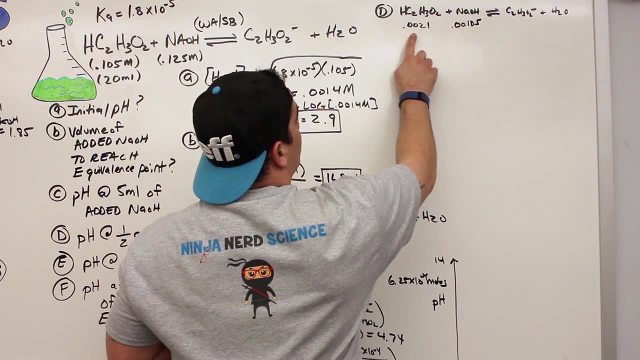 I'm going to get .00105.. So I'm going to get .00105.. So now, what I'm going to do is I'm going to subtract .00105 from him. So I'm going to subtract .00105 from him. 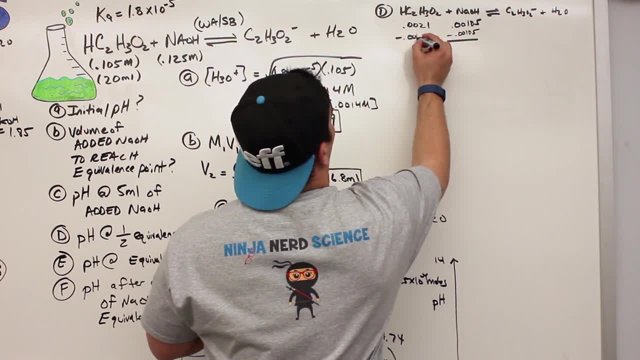 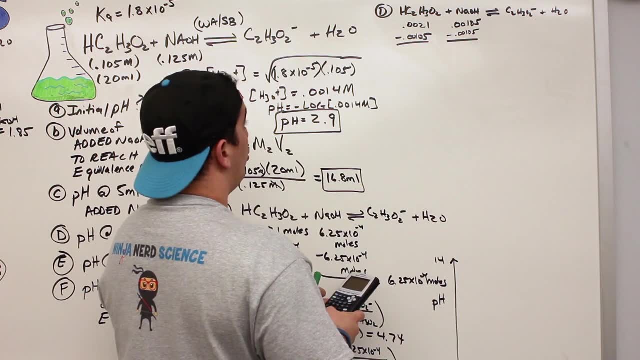 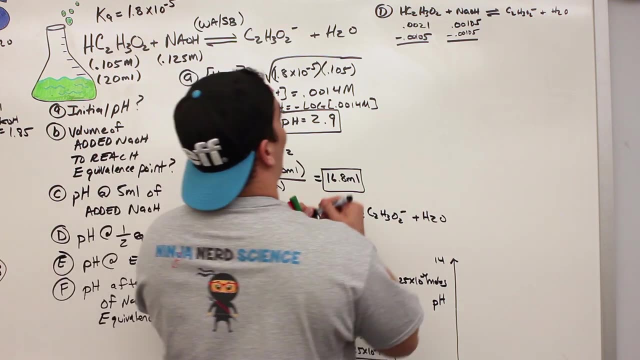 And now I'm going to subtract .00105,. okay, What do I get then? If I take .0021 and I subtract .00105,, I get .00105, right, .00105 moles. And then, remember, what do I get out of this one? 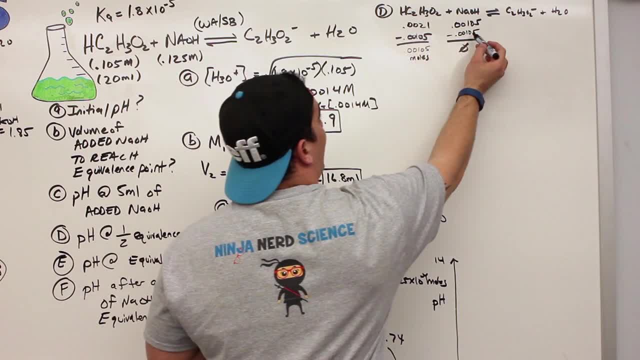 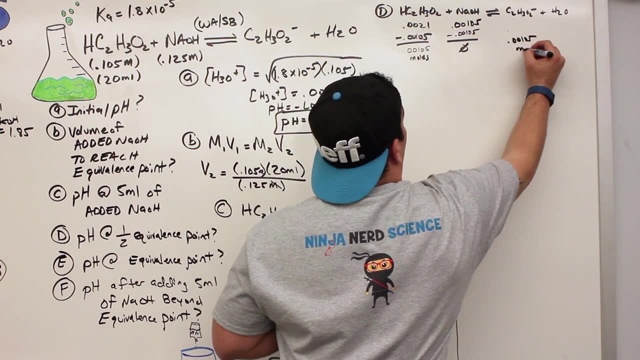 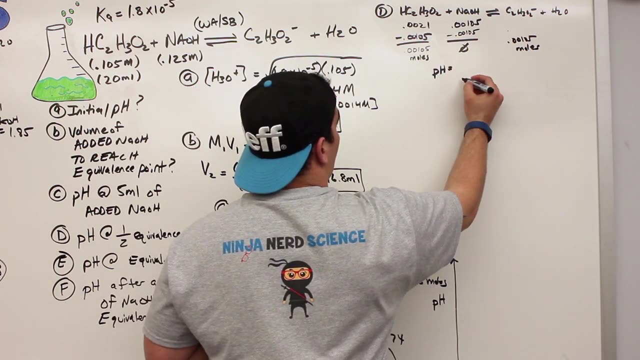 Zero, But .0015 moles of acetic acid reacts with .00105 moles of sodium hydroxide and produces .00105 moles of acetate. If I plug this into the Henderson-Hasselbalch equation real quick, pH is equal to the pKa. 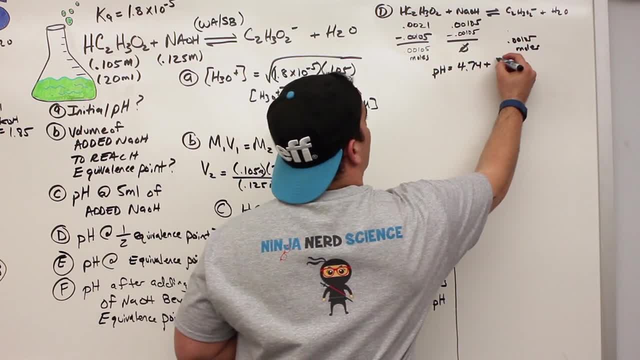 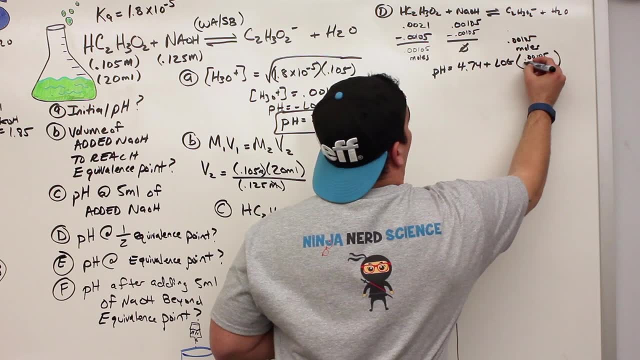 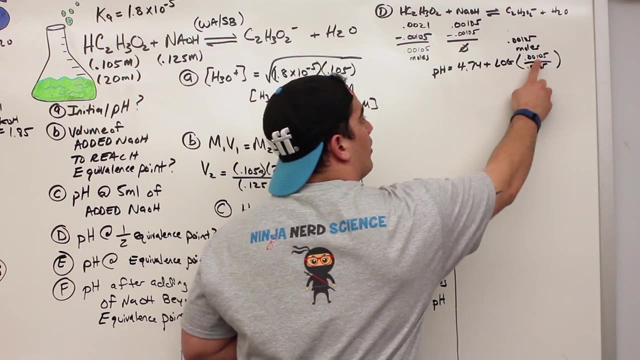 which was 4.74, plus the log of my base, which is again .00105,, over the moles of my acid, which is .00105.. What is that going to be? One. What's the log of one Zero. 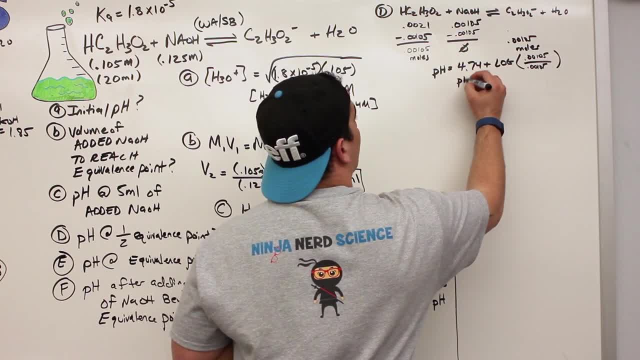 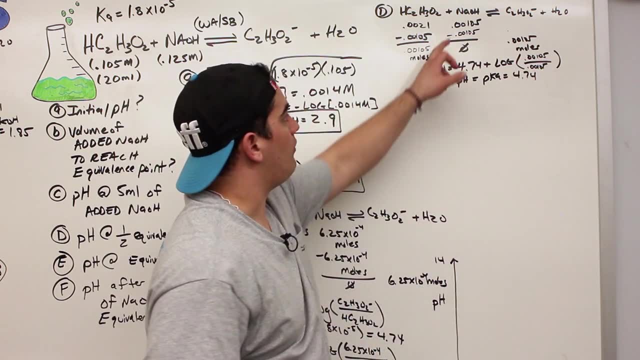 So pH equals the pKa Zero. Okay, and the pKa in this case is 4.74.. Now here, let me come back here. You guys are probably wondering how the heck did I get .00105 besides dividing it? 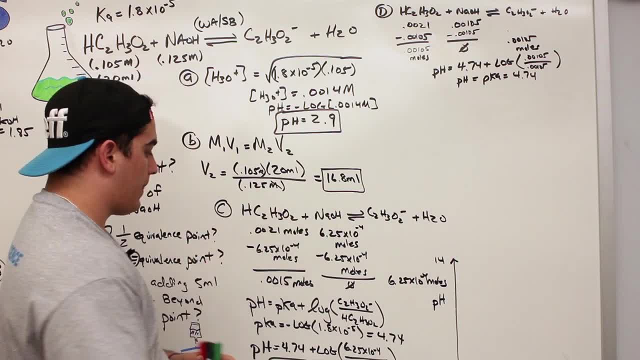 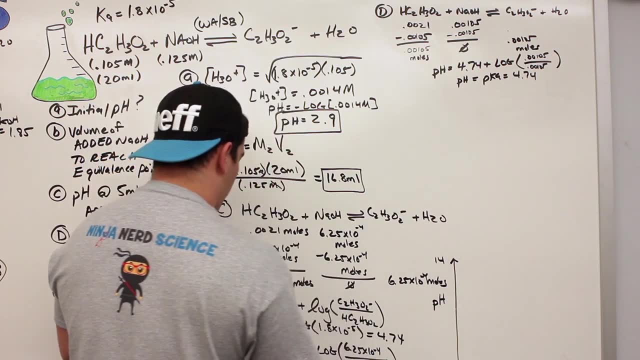 What was the volume that it took to get us to the equivalence point? 16.8, right. So let's take that and half it. So what's 16.8 divided by 2? That is 8.4 milliliters, which is .0084, right. 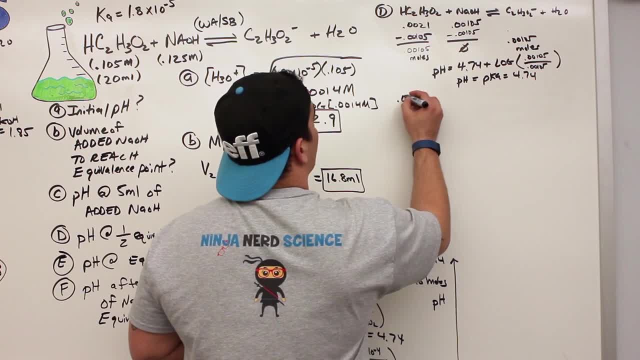 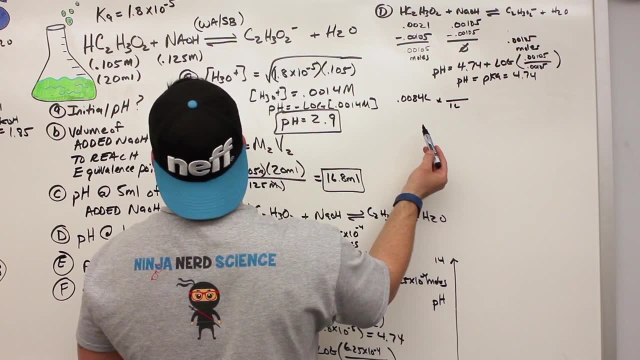 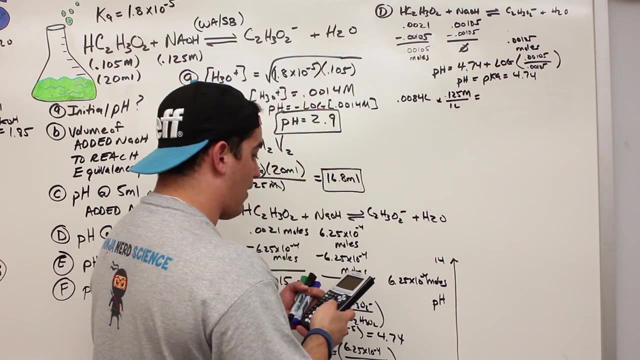 So it's .0084 liters. So if I take that and half it, what's 16.8 divided by 2?? I take .0084 liters, right, and I multiply that by whatever the molarity was of the sodium hydroxide, which is .125 molar, I should get .00105.. 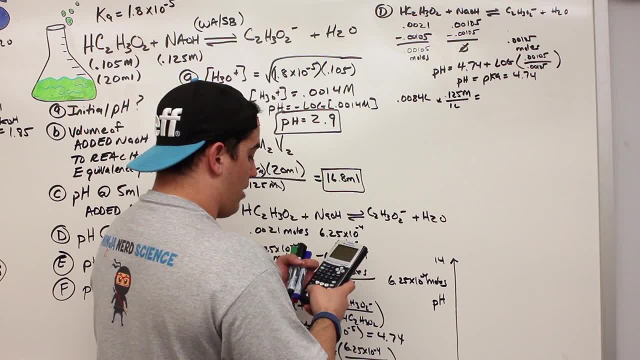 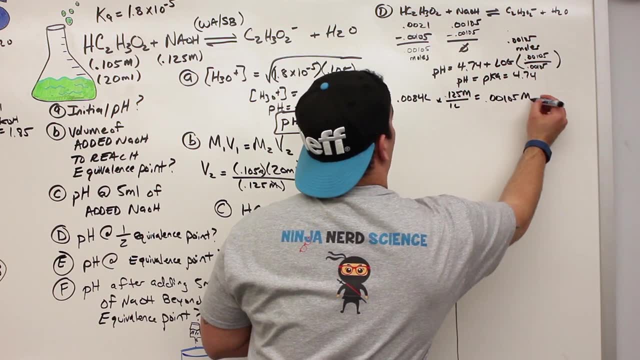 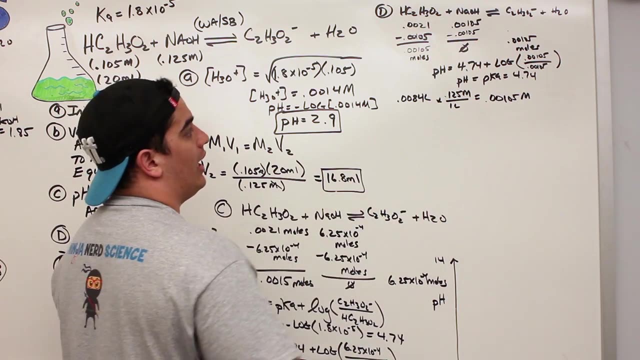 So let me do that real quick and multiply that by .125, and I get .00105, okay, So that's how I got that. I took whatever the volume took to get me to the equivalence point and I half it. That's half the equivalence point. 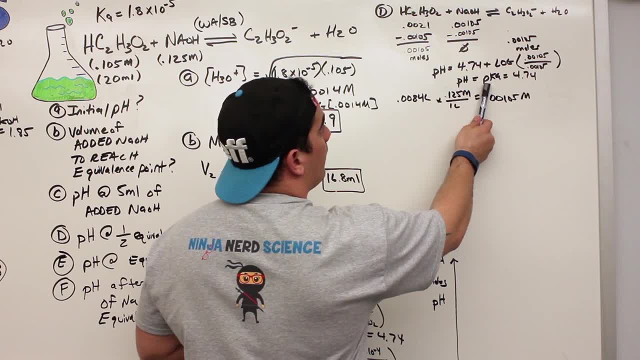 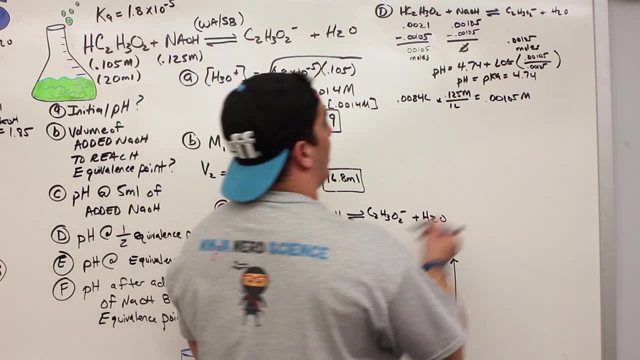 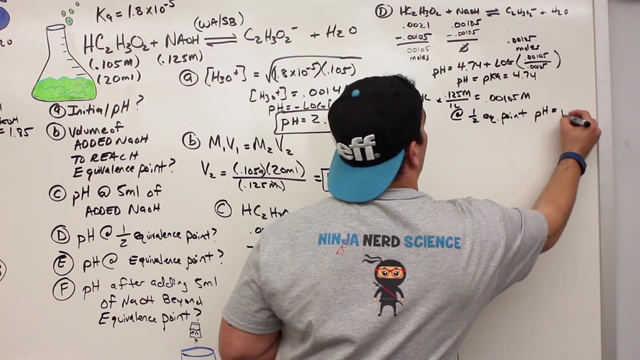 And at that point in time, just remember, stick this into your cerebral cortex and remember it. At the half the equivalence point, the pH is equal to the pKa. Make it a quick, easy problem, okay. So again, at half the equivalence point, at half equivalence point, pH equals pKa. okay, 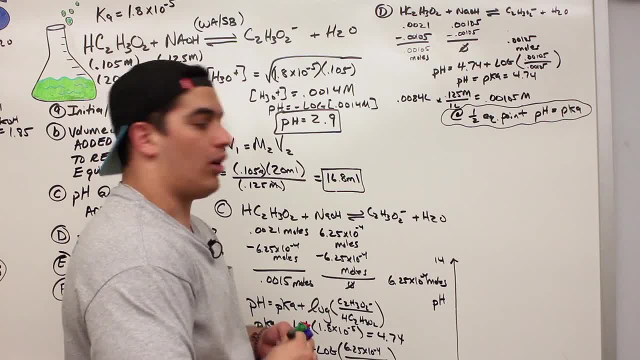 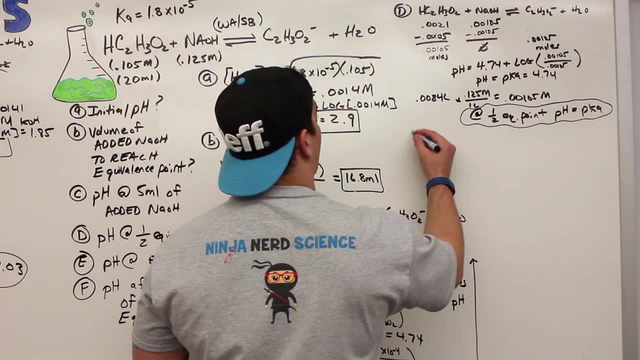 This is a super, super important one. quick, easy points to get out of this one, Okay. Next one: E pH at the equivalence point. all right, So let's go ahead and E here. At the equivalence point. the moles of my acid and the moles of my base have to equal. 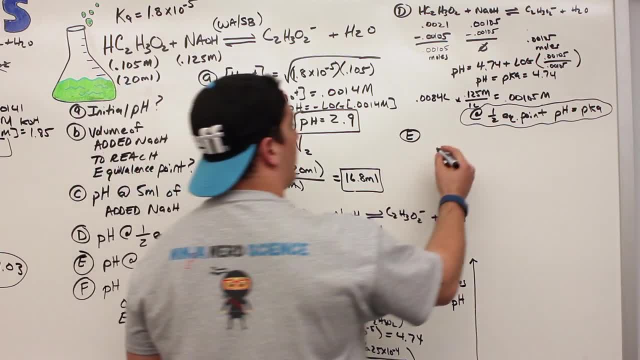 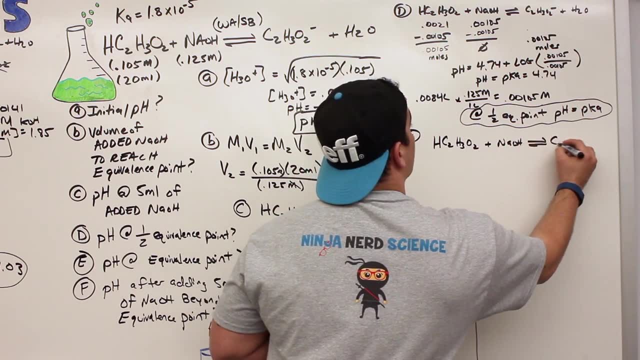 each other. Okay, So then, if that's the case, then let's write out an equation here: HC2H3O2 plus sodium hydroxide yields C2H3O2 negative and water. What's the moles of N that I started with again? 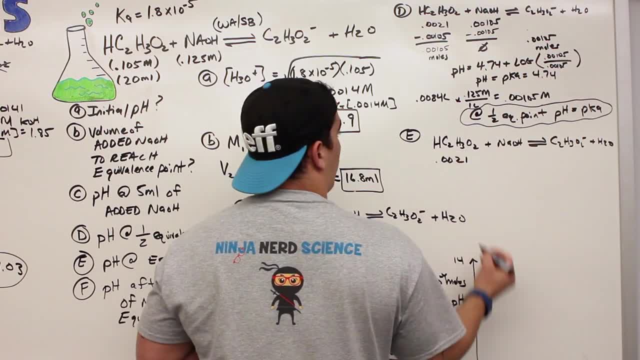 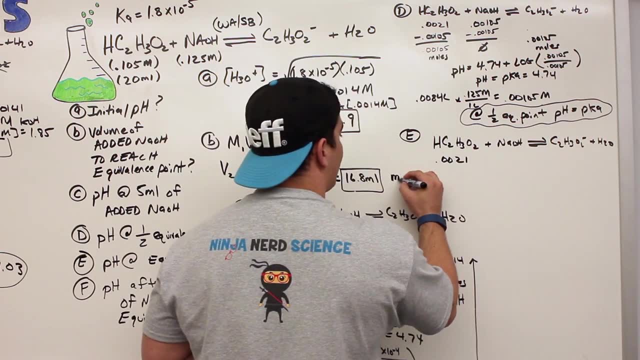 Okay, So I started with 0.0021 moles, and if I'm at the equivalence point, what does that mean for my sodium hydroxide? He's also equal, because that's what I said. Remember moles of acid. I'm going to put: moles of A equals moles of B, which is base. 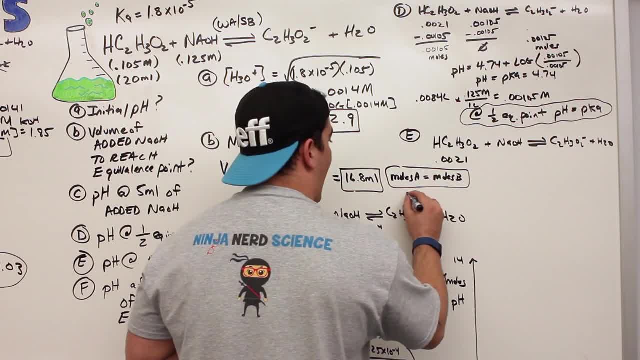 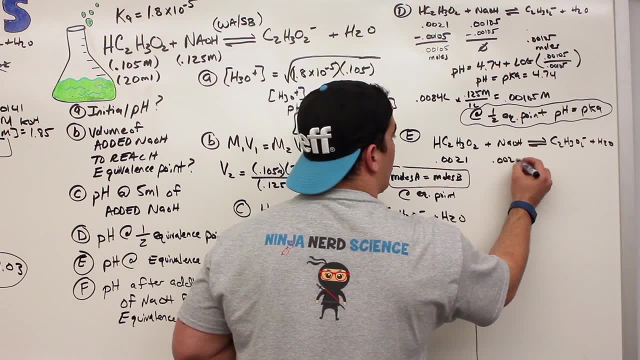 That's that thing that we need to remember at the equivalence point. at equivalence point, So this guy's 0.0021, he's also 0.0021.. If I subtract these two, so I'm going to erase this now. 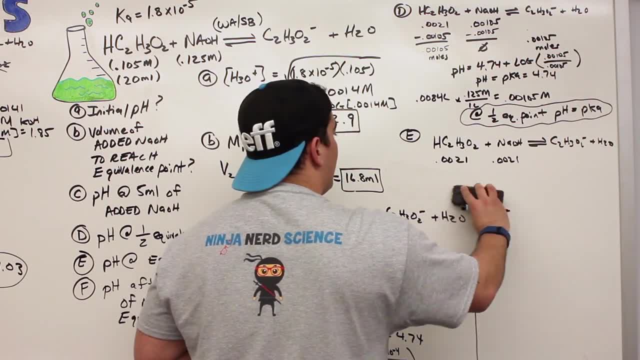 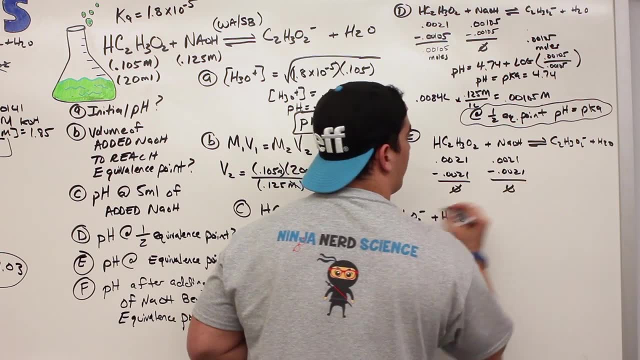 Now that we know this concept here, If I subtract the difference between these two, what am I going to get? 0.0021 minus 0.0021, I'm going to get 0 for him, 0 for him. 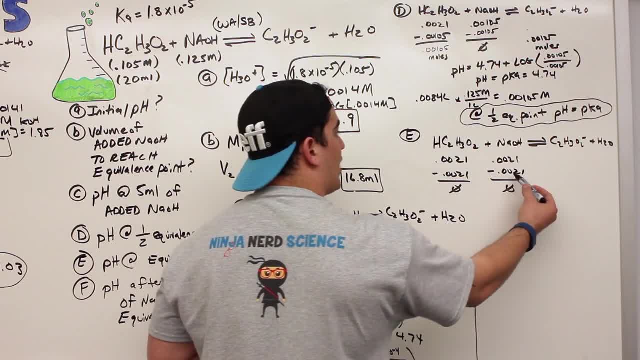 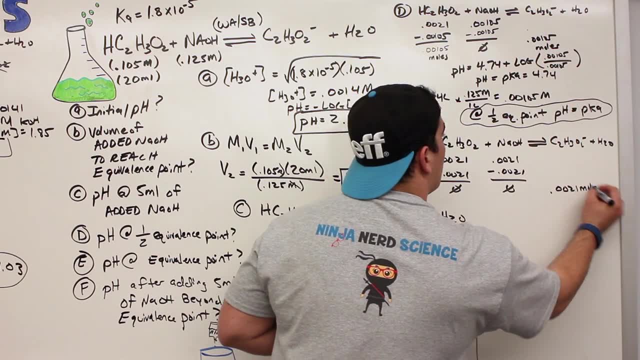 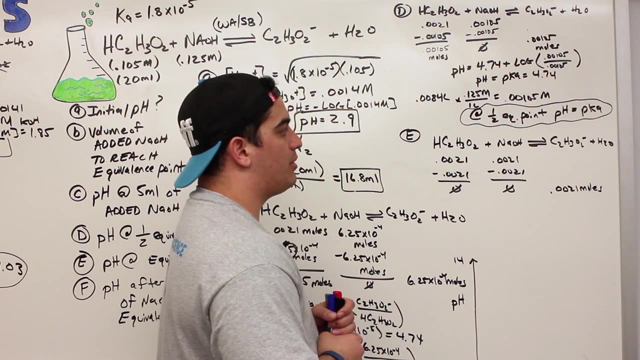 But again, 0.0021 moles of acetic acid reacts with 0.0021 moles of sodium hydroxide and produces 0.0021 moles of acetate. Okay, So now all we have left sitting in this beaker. 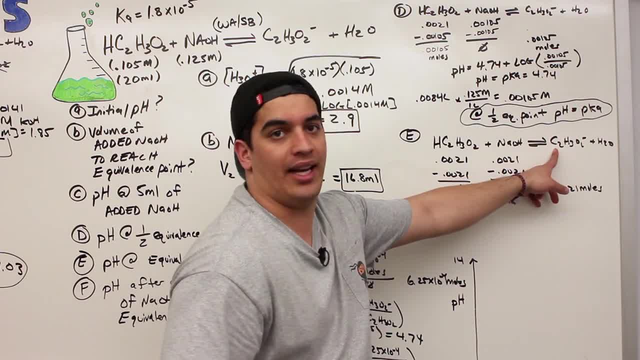 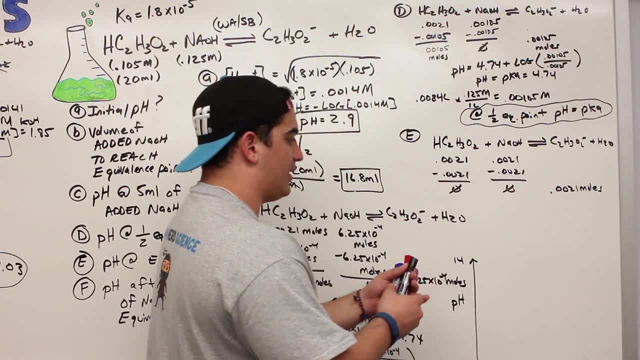 Is some basic solution. right here We have some acetate, this weak base, over here. That's the moles of the weak base. Now we have to figure out how much volume is this acetate sitting in? Okay, Well, what was the initial volume of the acetic acid? 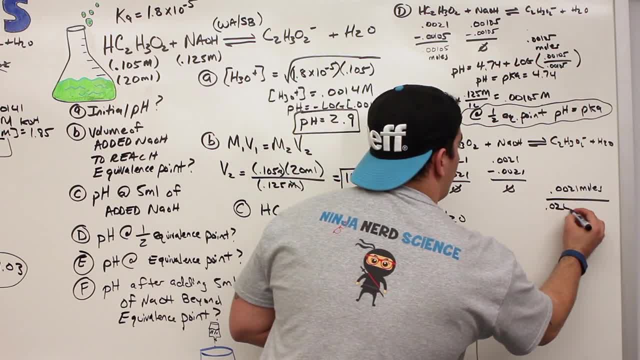 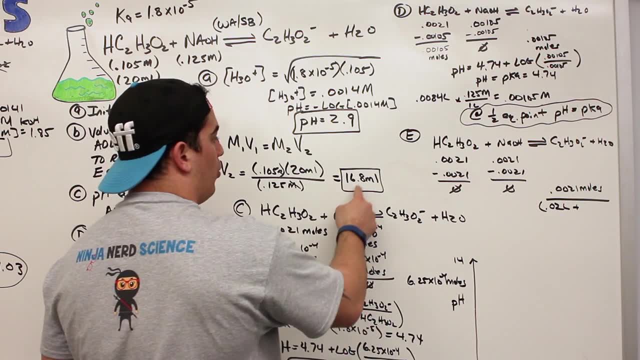 It was 20 milliliters, which is 0.02 liters. And how much volume did it take for me to be able to get to the equivalence point? It took 16.8, but we needed a liter. So it is 1, 2,, 3.0168.. 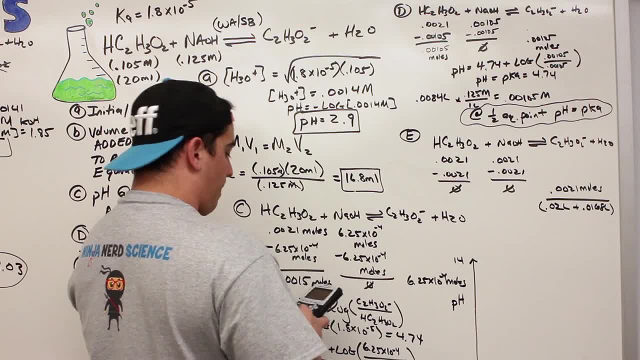 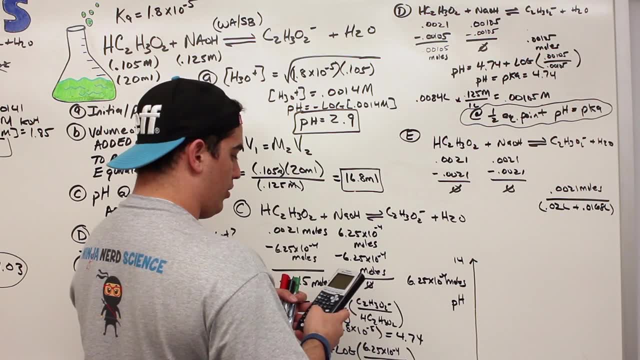 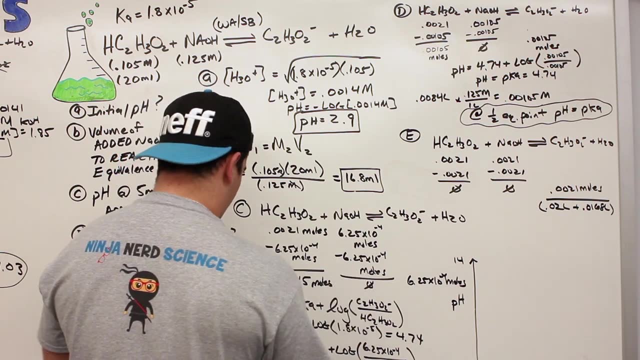 I'm going to go ahead and divide that right there. So let's take this one: 0.0021, and I'm going to divide this by 0.02 plus 0.0168.. And I'm going to get 0.057.. 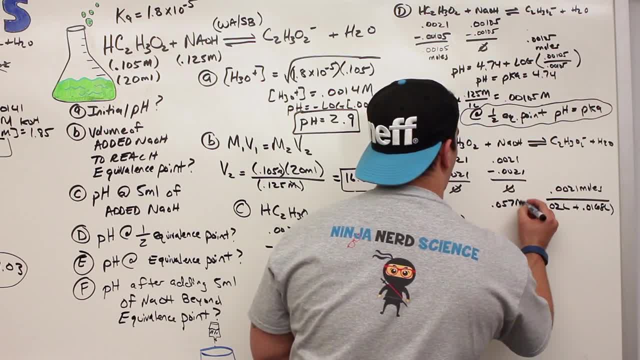 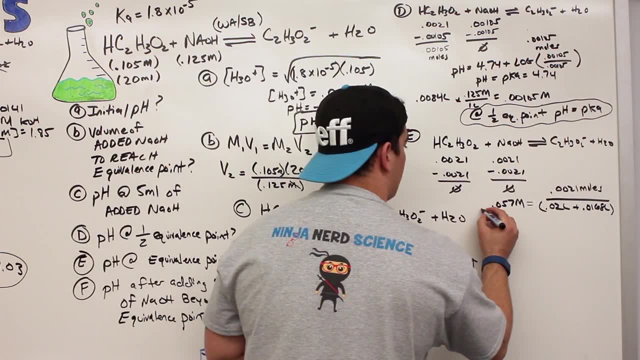 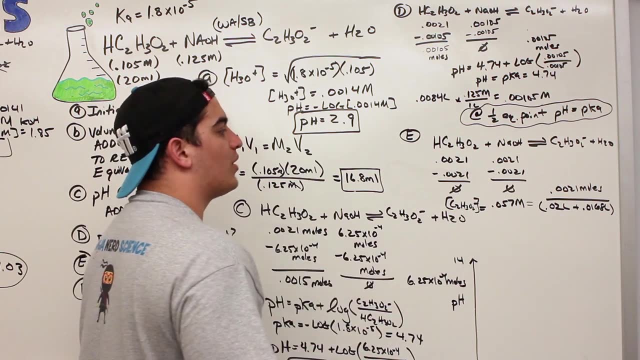 So, out of this, the molarity that I'm left with is 0.057 molarity. And who is this for? This is equal to my conjugate base, right there? Okay, C2H3O2 negative. Well, he's acting as our weak base, right there. 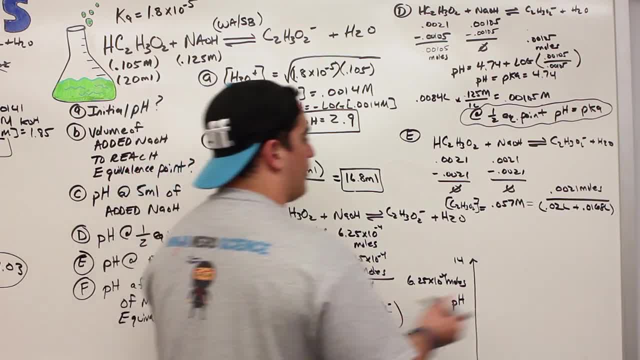 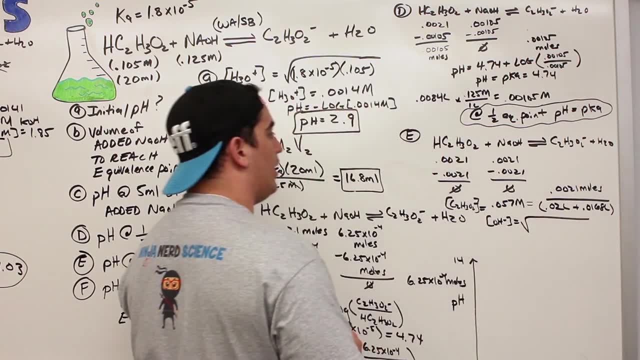 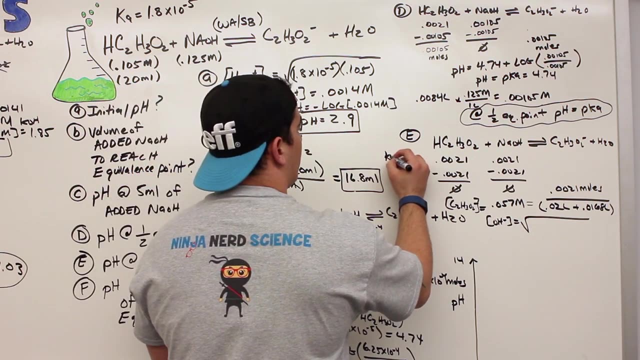 What's the weak base formula, guys? The weak base formula is hydroxide ion concentration is equal to the square root of the KB. Now I need the KB. I was given the KA. Remember that formula? What was it? KW divided by KA is KB. 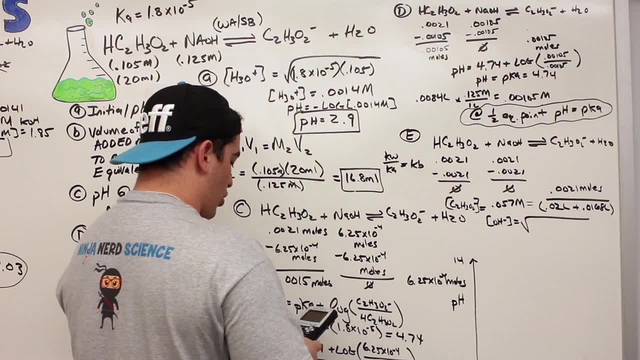 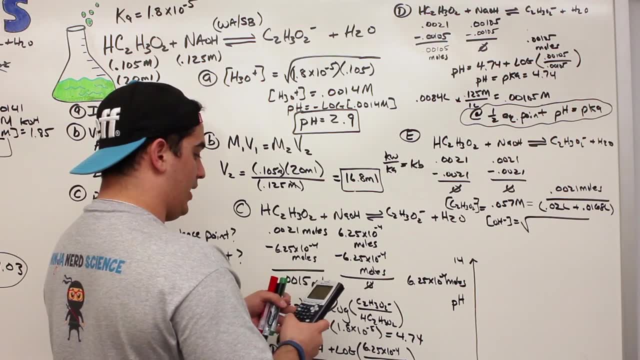 So what do I need to do then? Okay, I need to take KW, which is 1.0 second e to the negative 14, and divide that by my KA, which is 1.8 second e to the negative 5.. 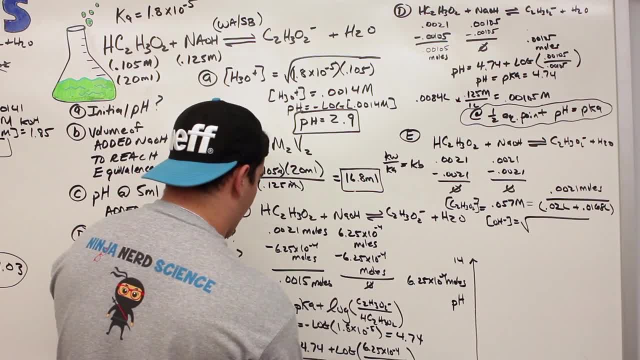 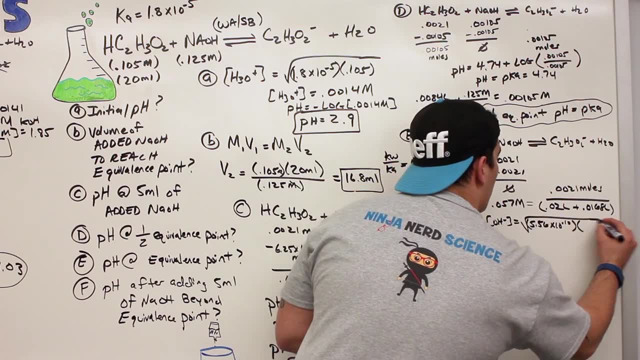 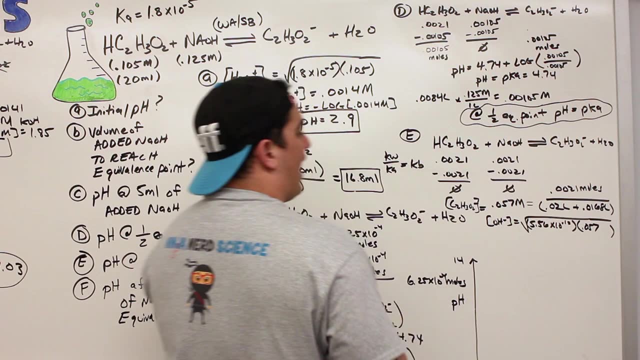 And I get 5.56 times 10 to the negative 10.. So 5.56 times 10 to the negative 10, multiplied by the concentration of my weak base here, which is 0.057.. And then, right after this, I'm just going to take the negative long. 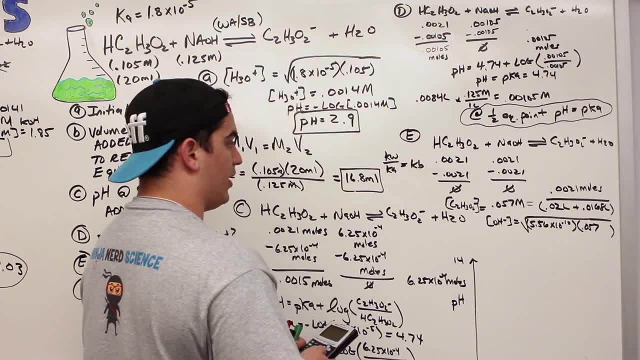 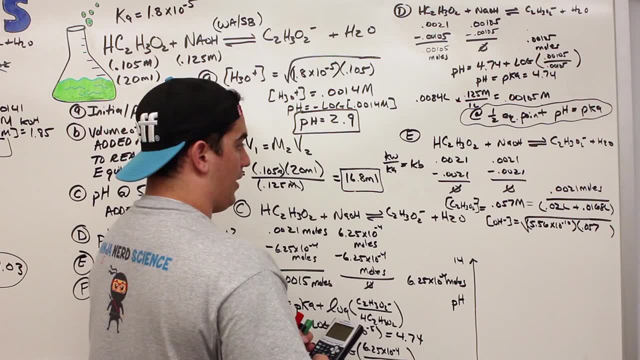 Okay, Okay, I'm going to take the log of that so that we can get our POH. So let's go ahead and do this real quick: Multiply that by 0.057.. Square root that. And then I'm going to go ahead and right away, I'm going to take the negative log of this. 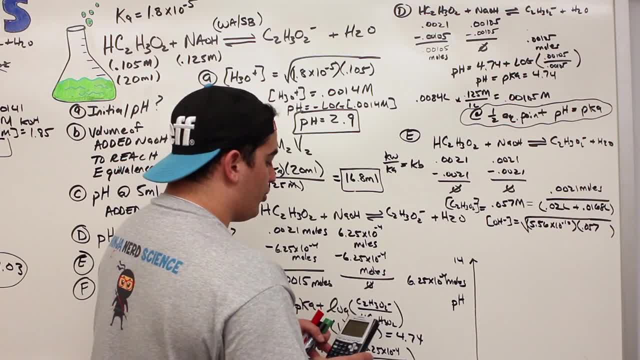 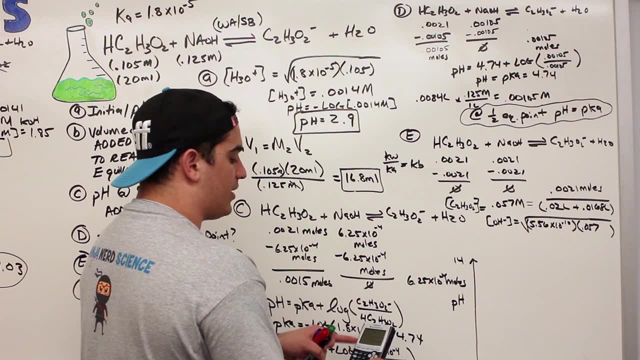 Okay, And you get 5.25.. And if you guys want to, you guys can write down the concentration I got. I got 5.63 times 10 to the negative 6.. But when I took the negative log I got 5.25 for my POH. 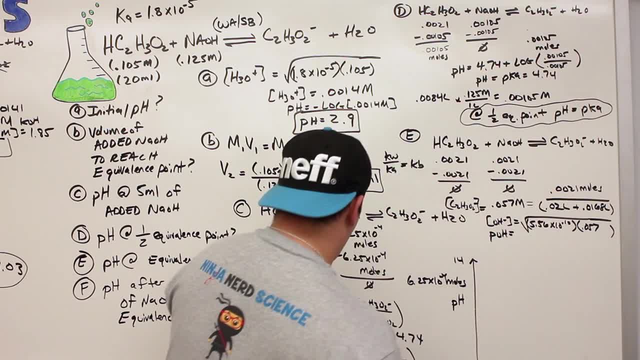 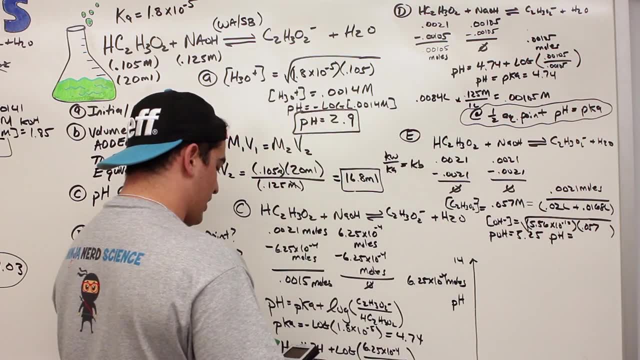 So POH is equal to 5.25.. And if I want the pH, I just take 14 minus that, right guys. So I'm going to take 14 minus that answer and I'm going to get about 8.75 for my pH. 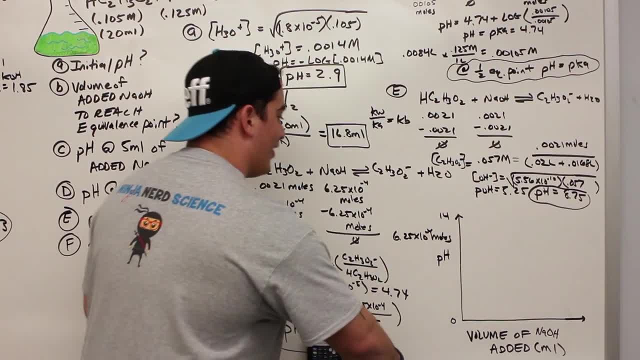 So we solved this one, All right, guys. So let's make some room for part F here. Definitely ran out of room on this one. We'll show you this titration curve on the over there on the left here in a second. 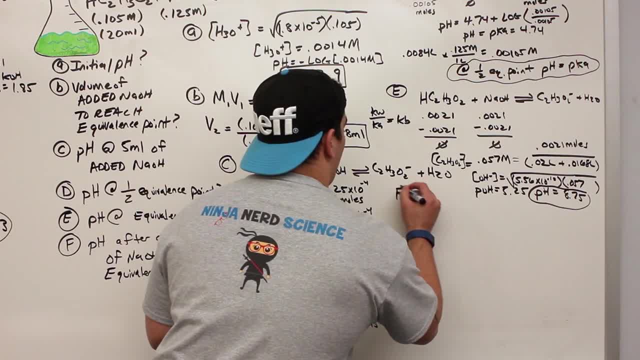 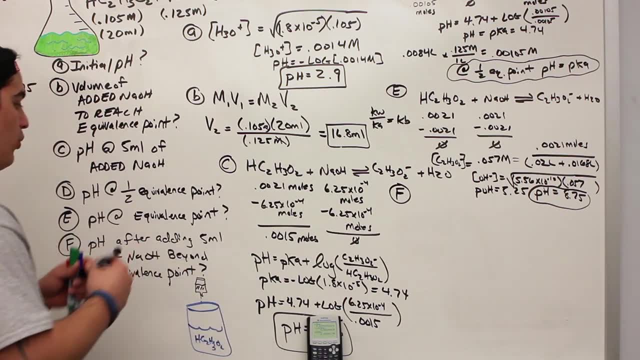 So let's make room for part F. So part F: What is? What is the question? It says pH after adding 5 mils of sodium hydroxide beyond the equivalence point. Okay, So what does that mean? then Let's write out this equation again. 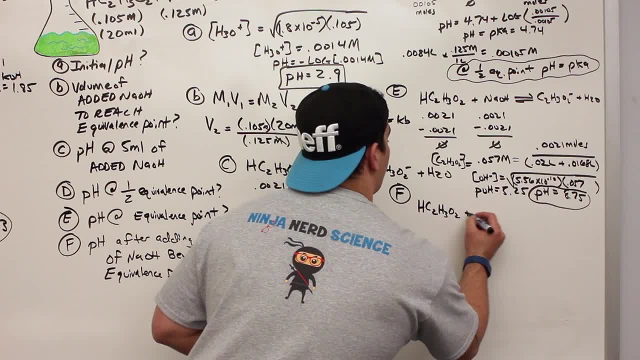 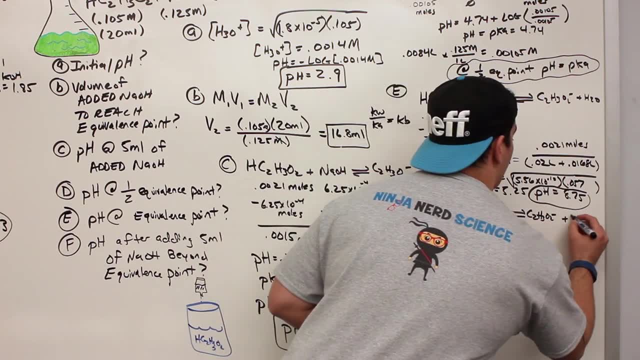 H, C2, H3 O2 plus sodium hydroxide, and then we get the C2, H3 O2 negative and then we get the water. Okay, Cool, So let's write out the moles that we had to him. 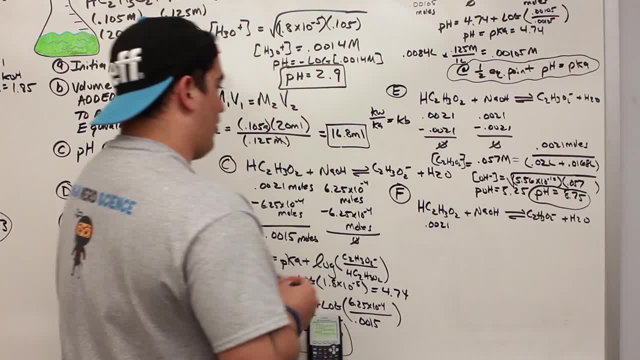 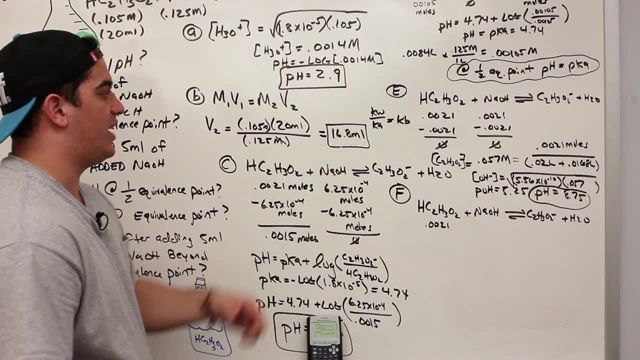 .0021.. Okay, But now look what we get here. We have 5 mils of sodium hydroxide beyond the equivalence point. What was the equivalence point? 16.8.. So I have to take 16.8 plus 5, because that's how much actual volume I'm adding. 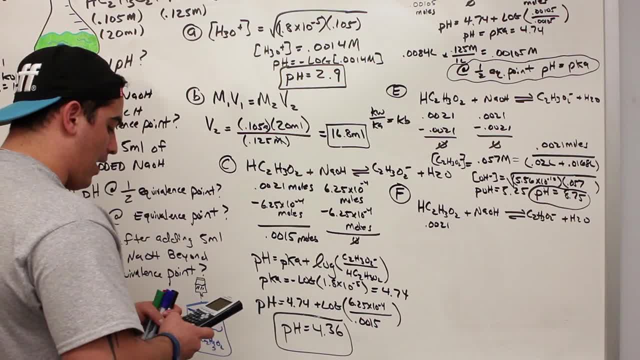 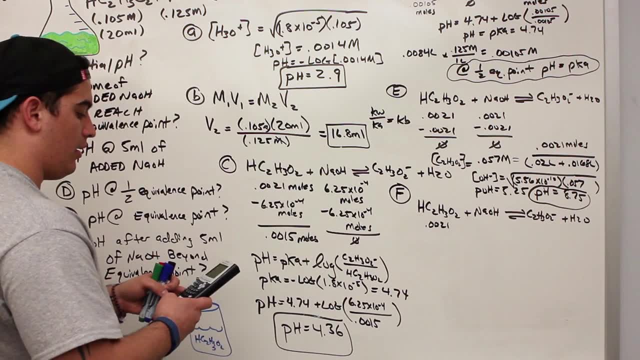 So I have 21.8 milliliters. so I'm going to divide that by a thousand so I can get it into liters, and then I'm going to multiply it by its molarity, which is 0.125.. What do I get? 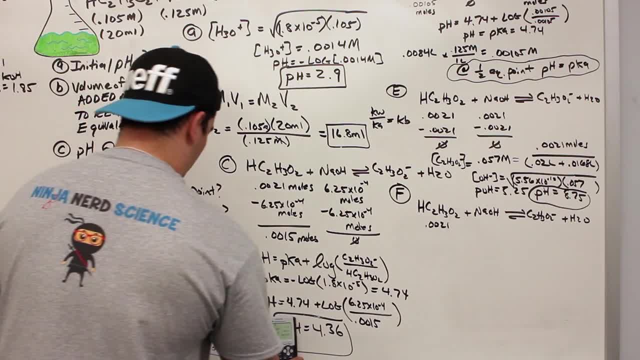 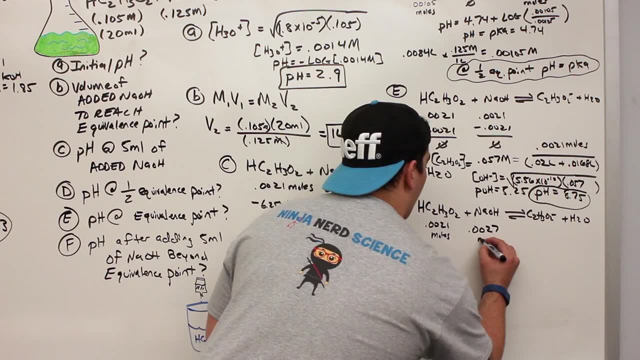 I get 0.0027.. Okay, Okay, I'm going to write that down here. So I get 0.0027 moles. So moles of this guy and moles of this guy. So now, what do I do? 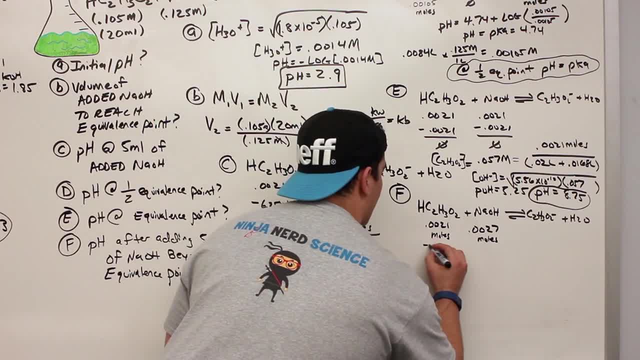 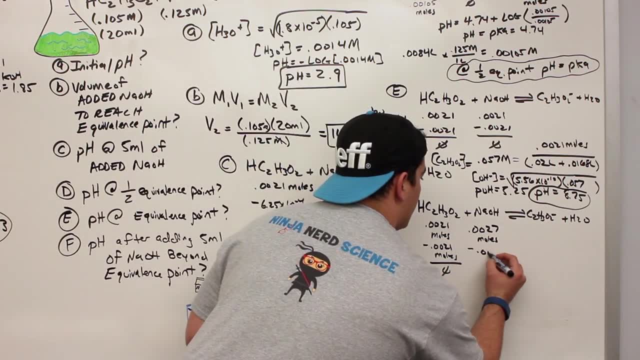 I subtract this guy, So I'm going to subtract out of this 0.0021 moles because he's in the lower amount, so all of him reacts and he reacts with this 0.0027 moles of the sodium hydroxide and 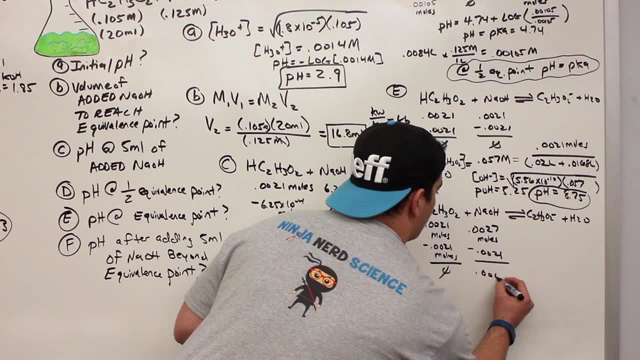 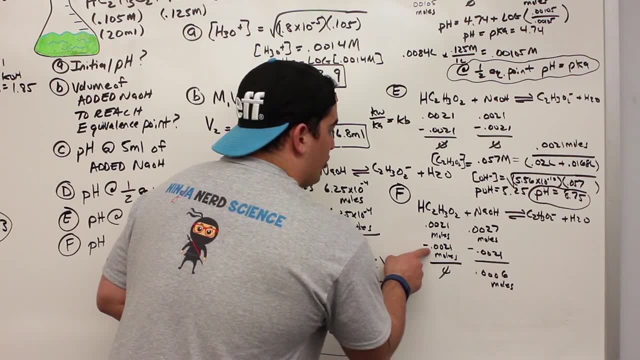 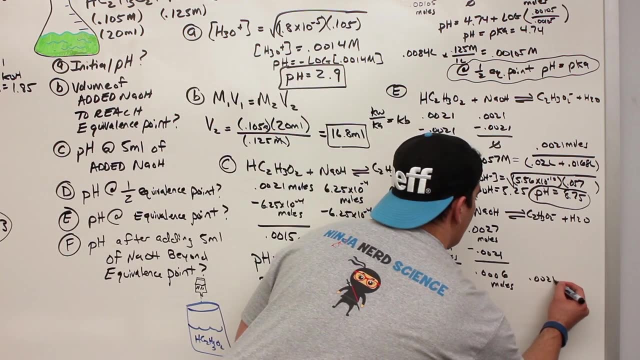 what does he leave? He'll leave 0.006 moles. Okay, Okay, Cool. So I get 0.0021 moles of the sodium hydroxide. But then what happens? 0.0021 moles of acetic acid reacts with 0.0021 moles of sodium hydroxide and produces 0.0021. 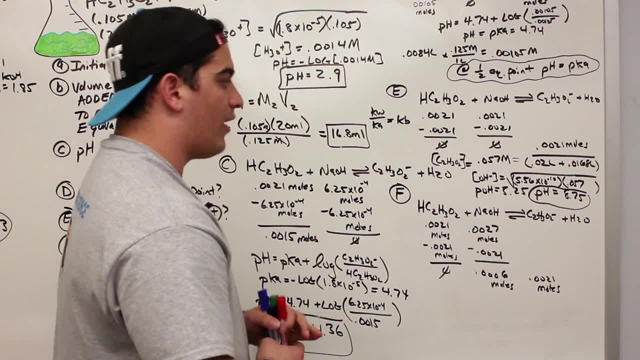 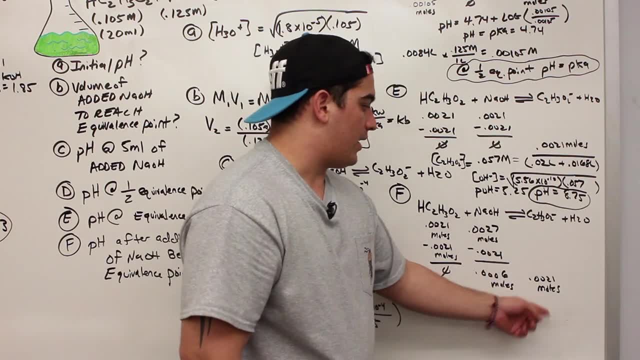 moles of the acetate. All right, This is weird. I never had this before. What do we do? I got sodium hydroxide, which is a strong base, and then I got acetate, which is a weak base. 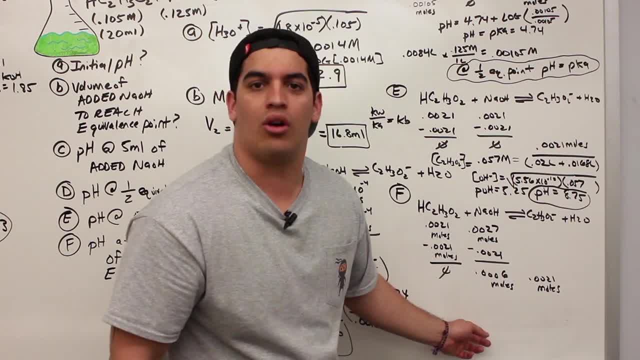 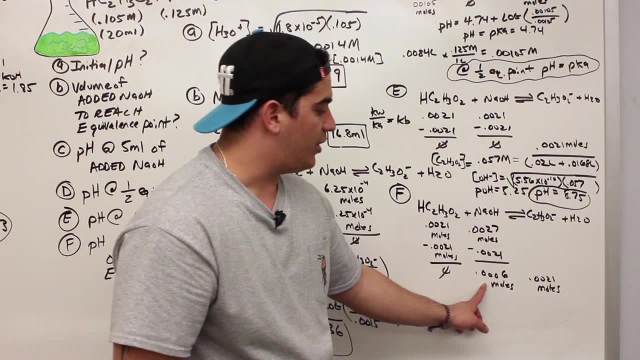 Who the frick wins. We always go with the strong, The stronger one. You don't care about this guy because he's weak. He's not really going to have as much of an effect as compared to the sodium hydroxide. 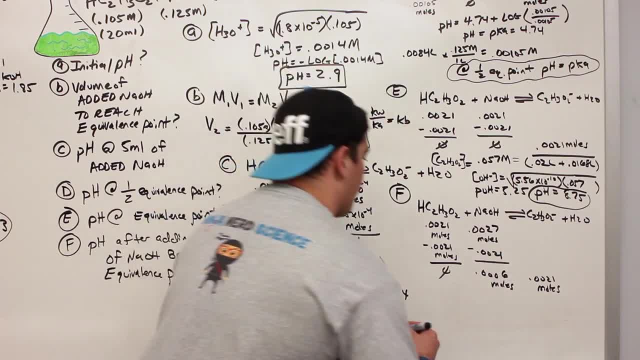 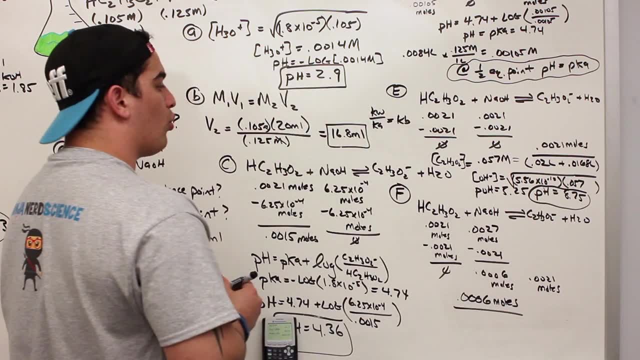 So he's the one that we really, really care about. So we're only going to look at his moles. So I'm going to take 0.006 moles of that sodium hydroxide. I'm going to put it over the total. 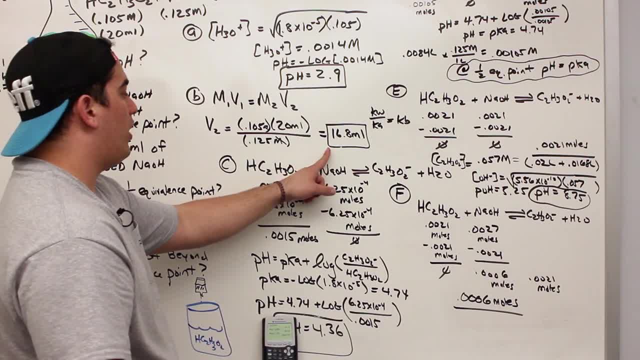 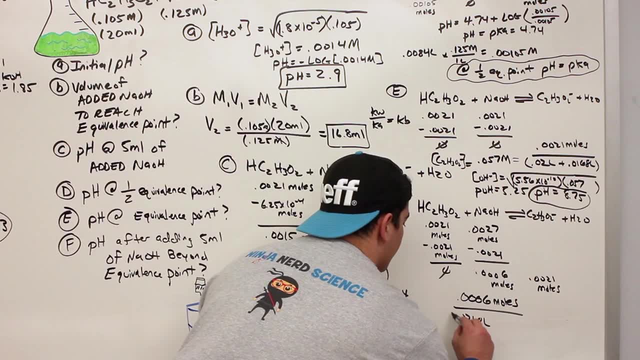 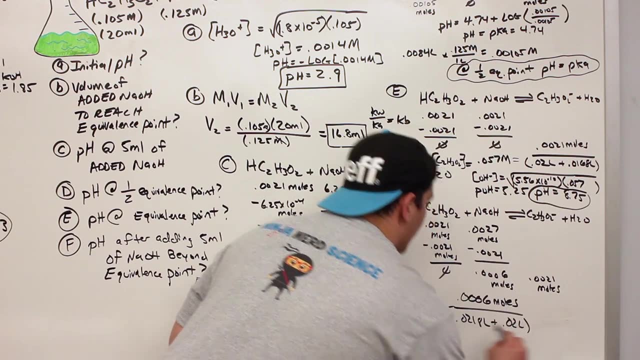 volume that we've gone to, which was 16.8 plus 5, which gave us 21.8 milliliters, which is 0.0218 liters. Okay, Okay, Okay. So that's the total volume of the acetic acid, which was 20 milliliters, which is 0.02 liters. 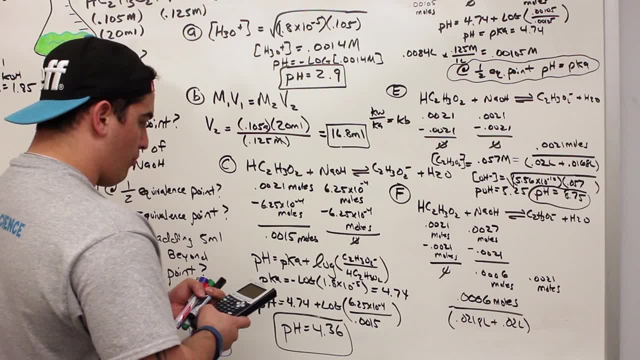 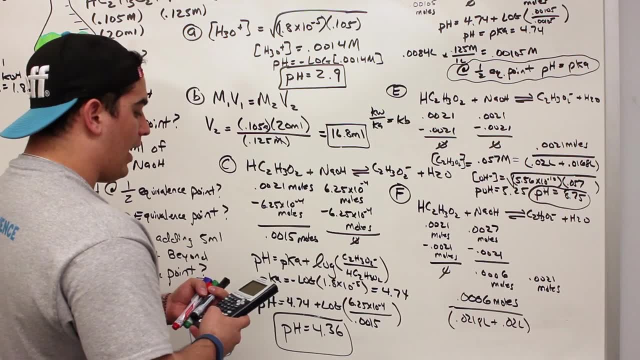 Let's get the molarity of this. So we're going to take 0.0006 divided by 0.0218, guys plus 0.02.. And we get a molarity of 0.0143.. I'll write it out for you guys, just to do that. 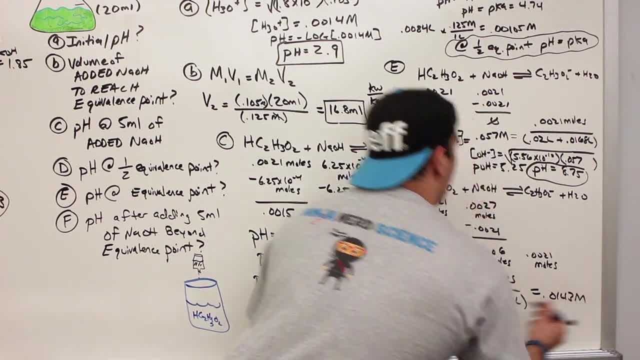 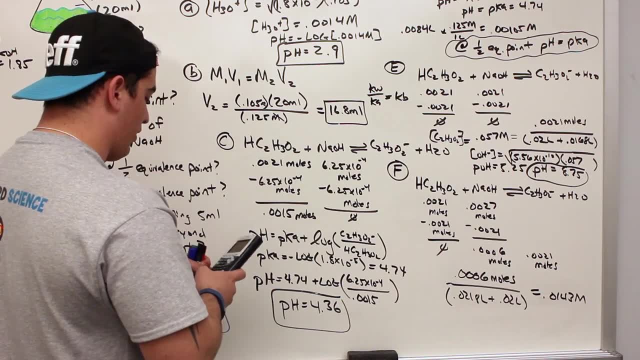 0.0143.. 0.0143 molarity. And then what's the rules? This is a strong base, Strong base, Strong base. We don't need a Ka, We just take the negative log of it. So negative log, second answer, and we get. what did we get? 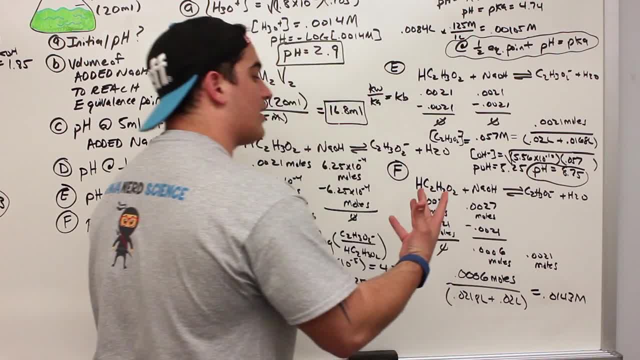 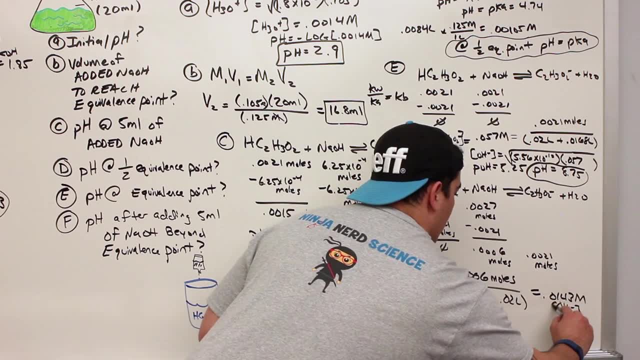 1.84, but this is the pOH. remember that, because we took the negative log of a hydroxide ion concentration here. okay, So we take the negative log. So again, this is hydroxide ion concentration, right here. 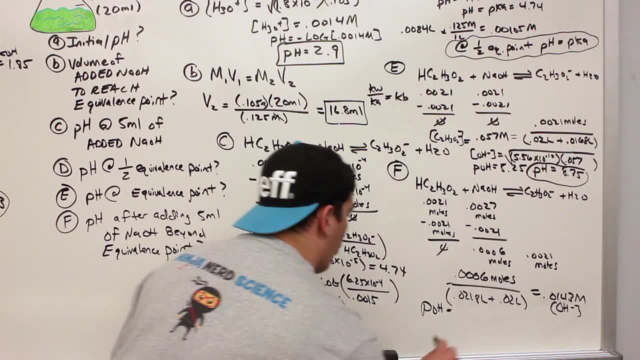 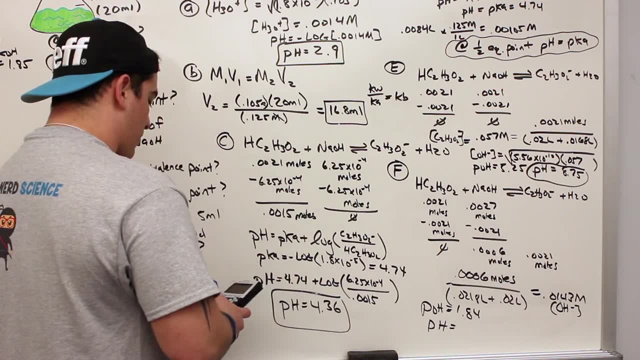 So what do we get? pOH is equal to 1.84, but if I do 14 minus that to get my pH, what do I get? 14 minus that, 14 minus that answer, and I get 12.2.. 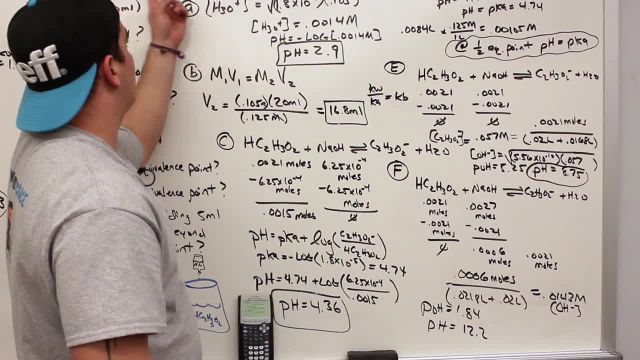 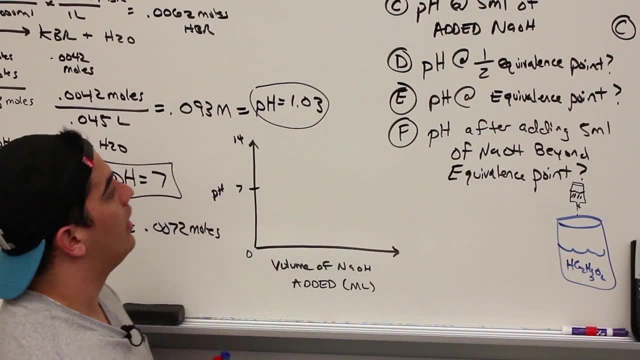 And that should make sense, guys, because look what we're adding. We're adding sodium hydroxide to a weak acid. It should be rising, okay, all the way up to go into the basic form. So again, if we look here at the titration curve, where did we start? 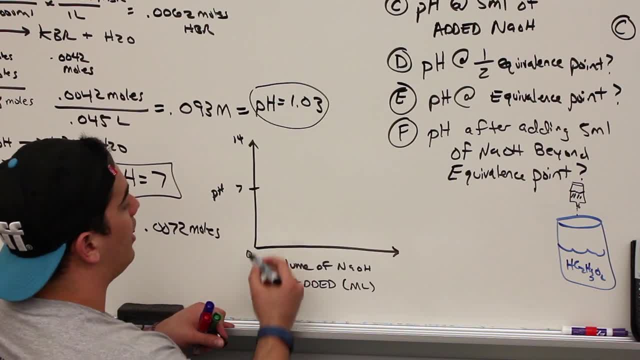 What was our initial pH? It was about 2.9.. So it's going to be a little bit higher than it was when we started with that actual strong acid, which was a lot closer to 0.. So we're going to probably start right around here. 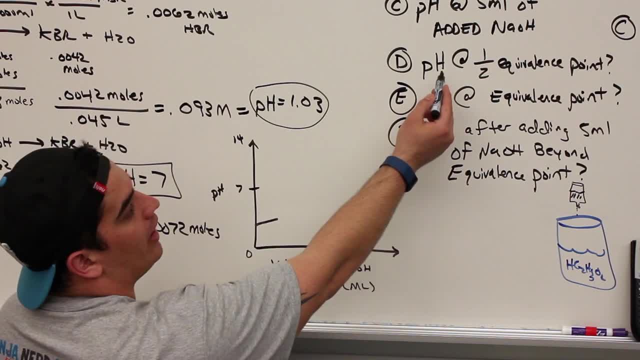 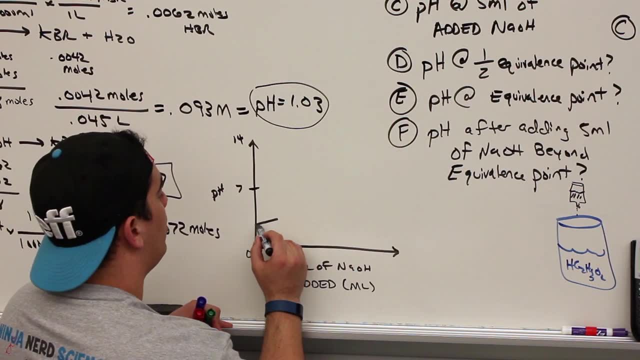 And then what happened? We have like this point, which is at half the equivalence point, right, So at half the equivalence point, the pH changed and it went up to about what it equaled the pKa, which was 4.74.. 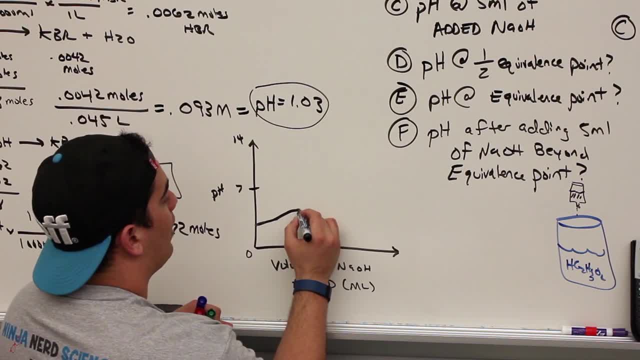 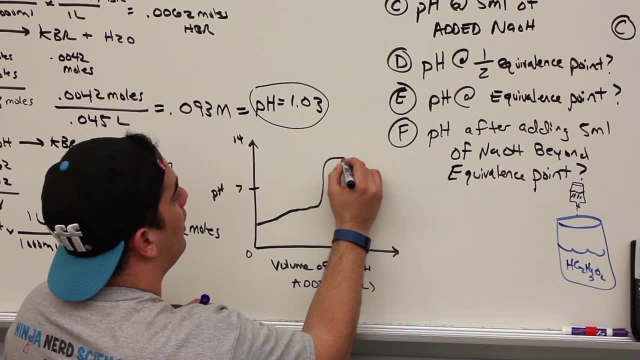 So you'll have this little like bump where it kind of like rises here and then look what happens Once you hit the specific volume that it takes to reach the equivalence point. so let's say it comes right here, boom, skyrockets up and then it goes over there, right? 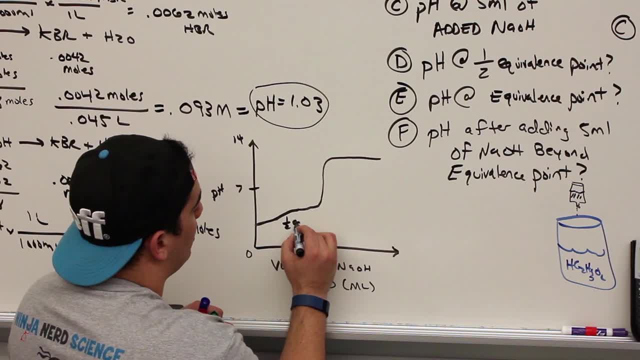 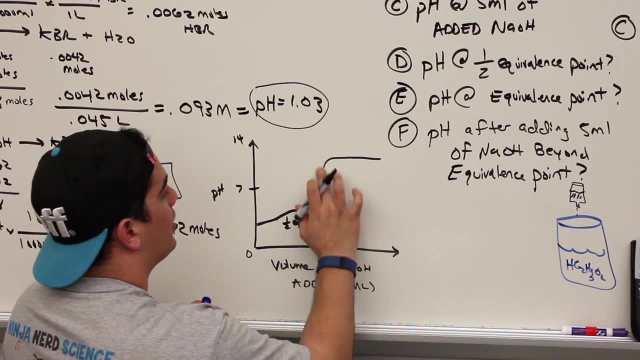 What was this point right here? This point right here is at half the equivalence point. Okay, So this point right here, where the moles of the acid and the moles of the base are equal. let's actually show this a little bit farther to the a little bit this way and more right. 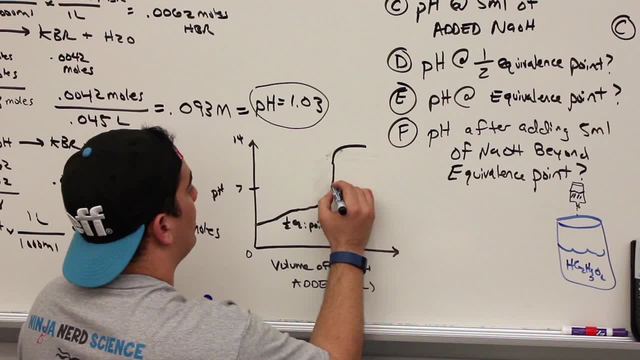 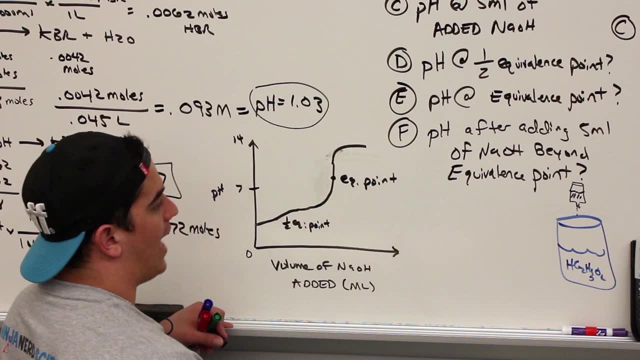 here Let's actually show it like that. I'm going to say it's right here, That's our equivalence point And that's where the moles of the acid and the moles of the base are equal. And then beyond this point is going to be beyond the equivalence point where we're working. 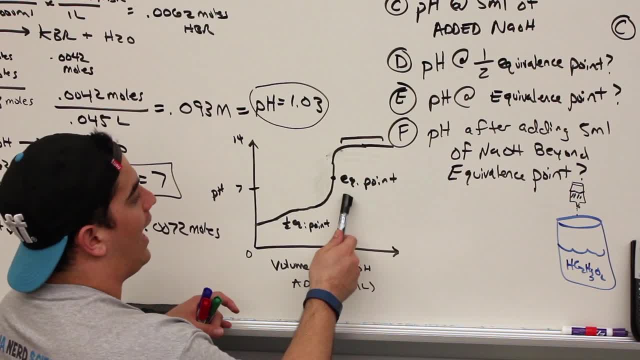 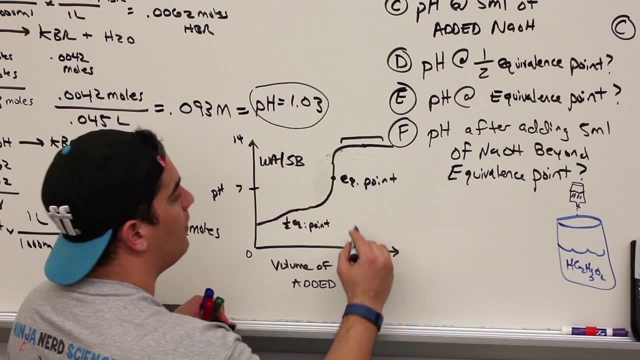 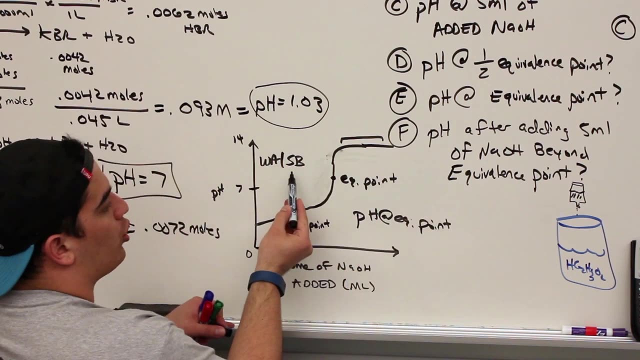 into base right? Why did I mention this At the equivalence point when you're doing a, what kind of titration is this? This is a weak acid. strong base titration. The pH at the equivalence point should always what's happening. I'm adding more strong base. 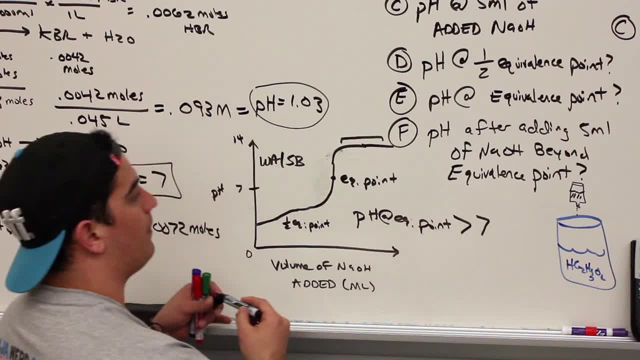 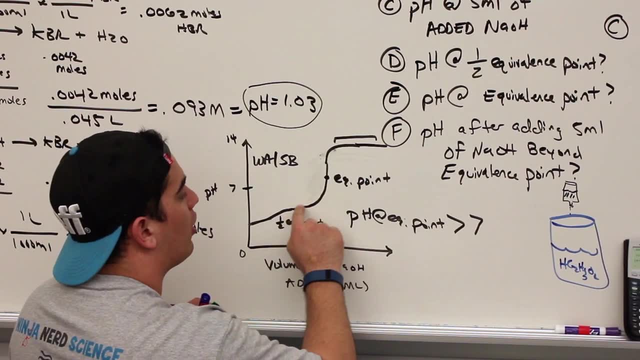 So the pH at the equivalence point should always be greater than seven. Okay, So that's giving us our titration curve. And again, half the equivalence point is this point right here where you might see a little bit of a, a little bit more of a larger rise as compared to the strong acid, strong base. 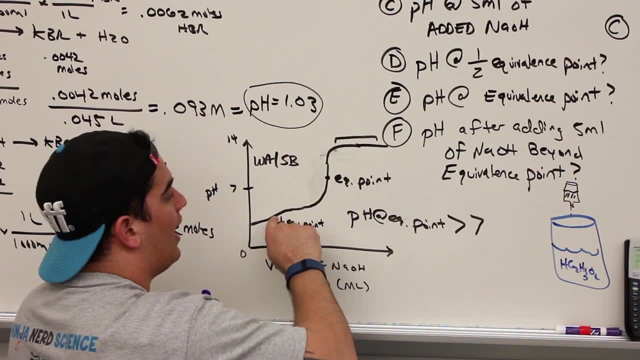 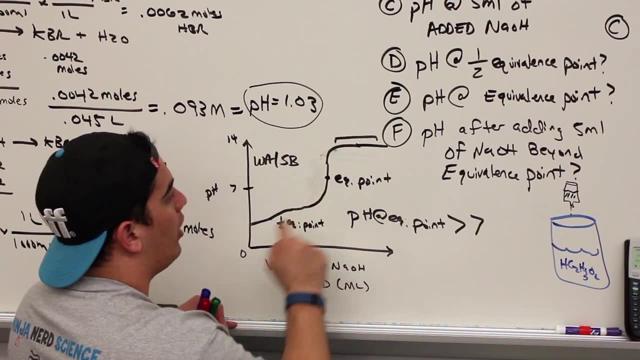 which is kind of a little bit more linear, More level, And then it has a drastic rise. This one kind of has a low, slow rise and then drastic rise. So we can half the equivalence point. Remember that. So just come here, half the equivalence point. equivalence point should always be greater.